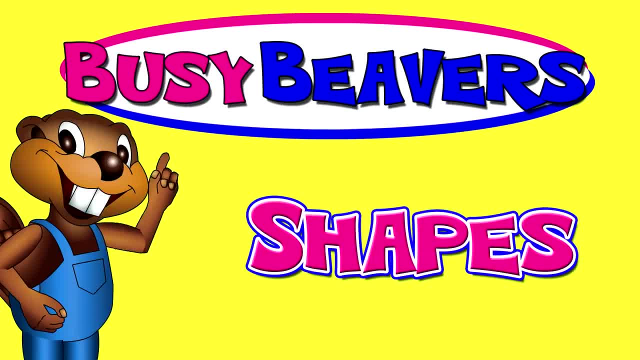 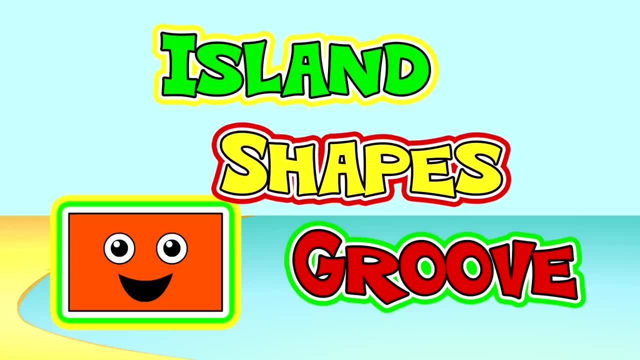 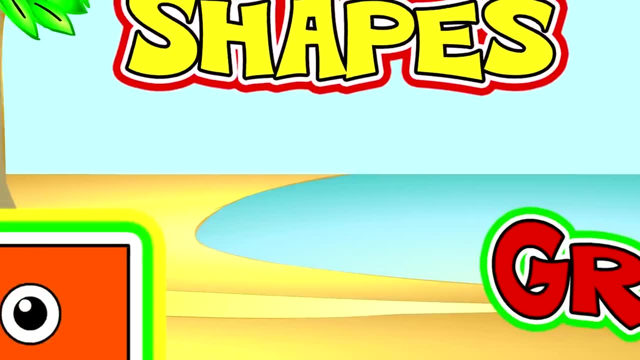 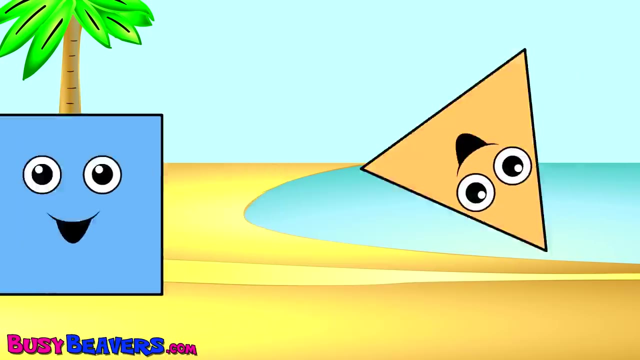 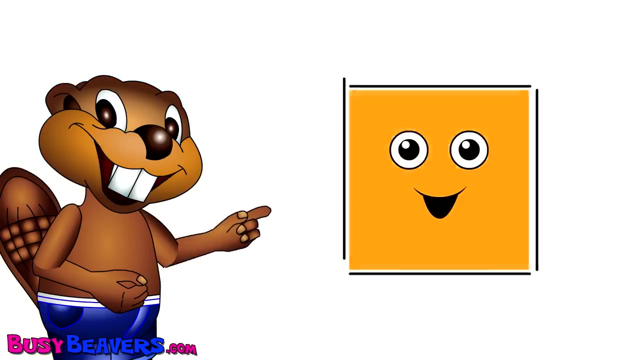 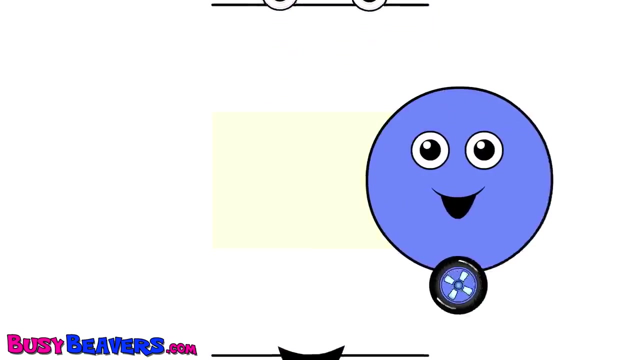 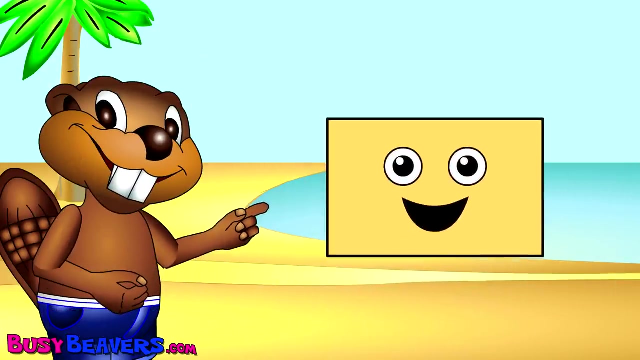 Welcome to the Busy Beaver's collection of shapes, songs, chants and lessons. Island Shapes- Groove Circle. square triangle- rectangle circle. square triangle rectangle- square triangle rectangle- square triangle rectangle circle. square triangle, rectangle circle. 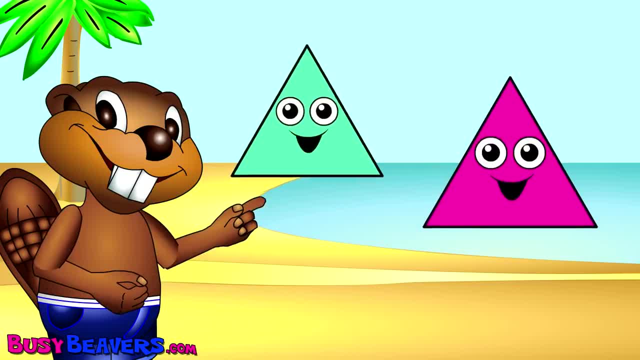 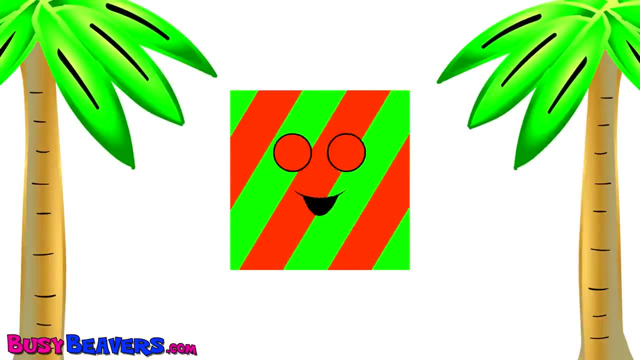 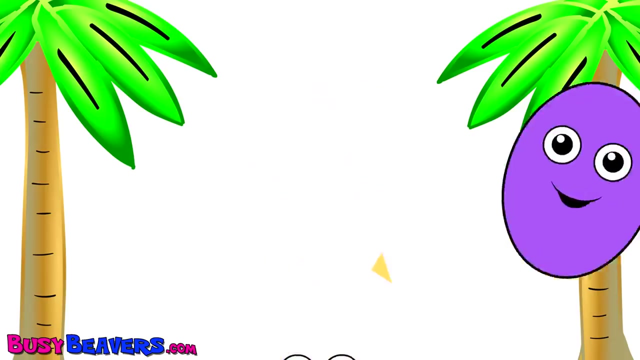 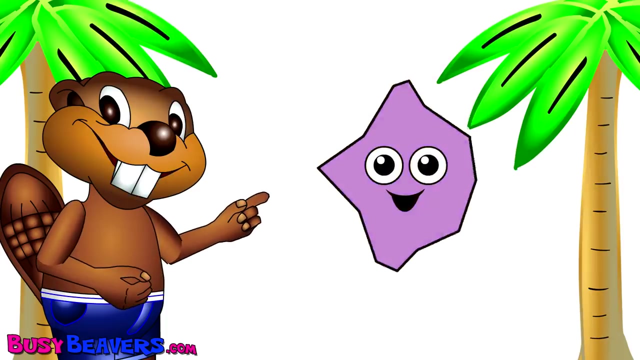 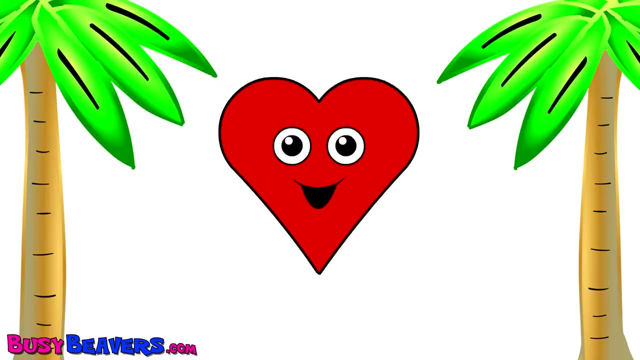 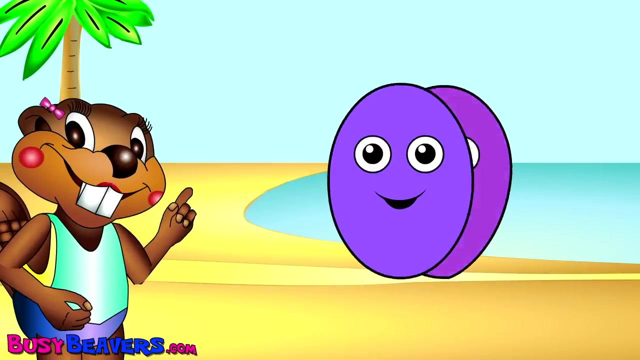 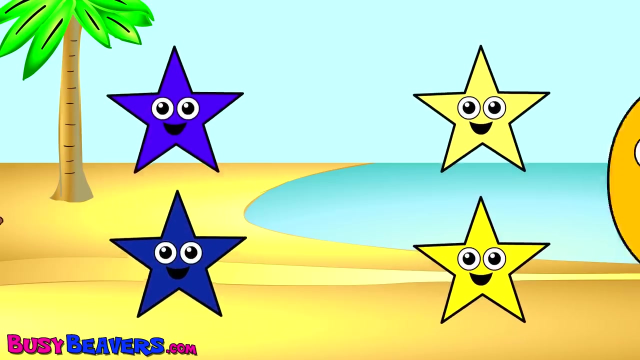 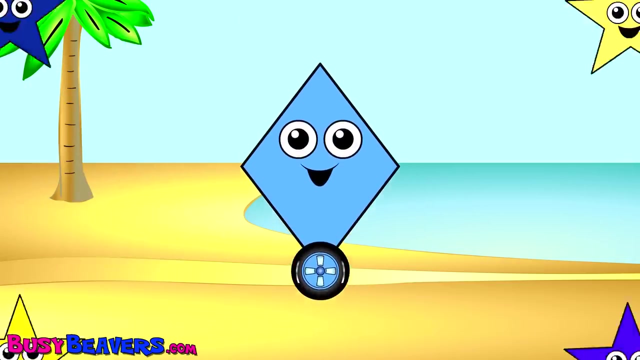 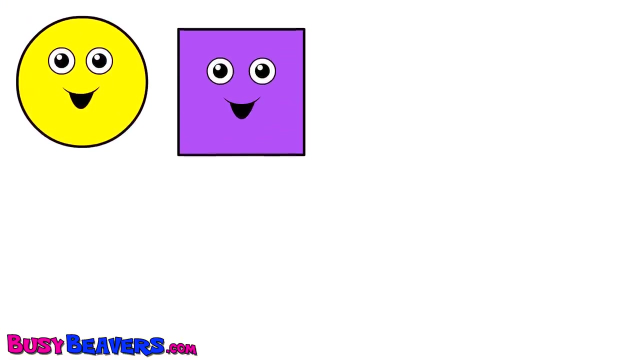 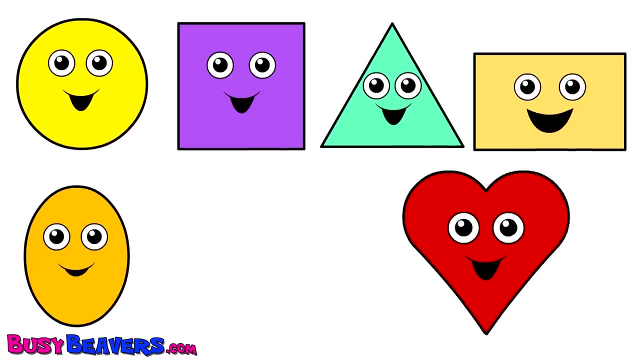 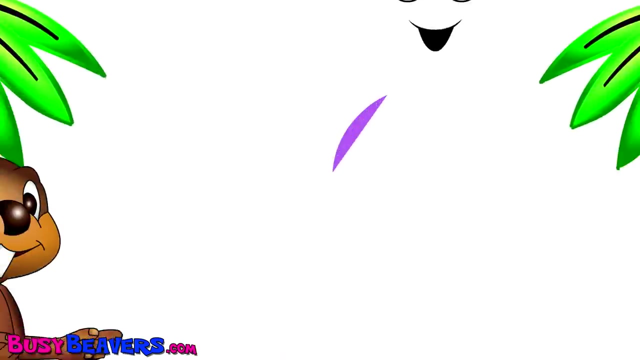 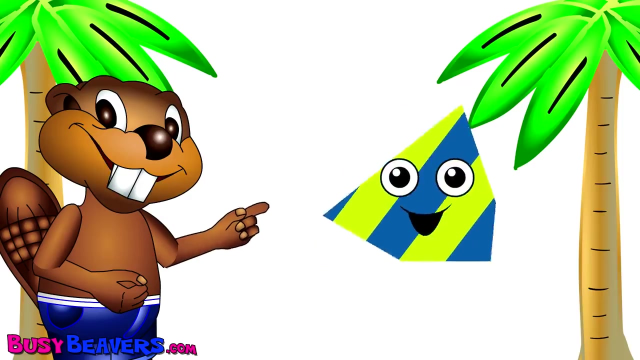 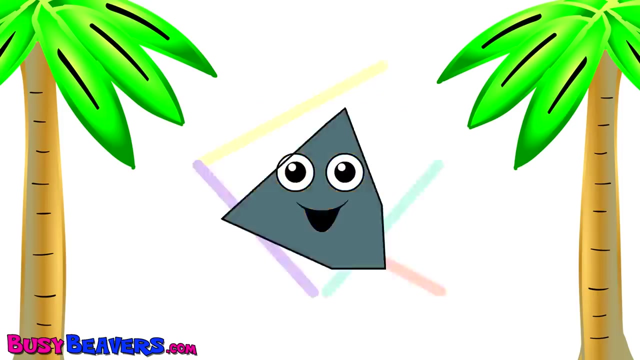 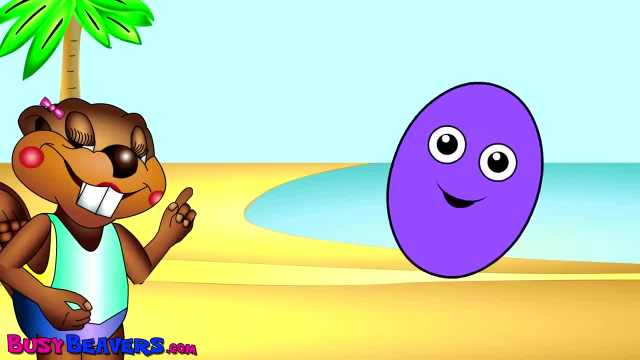 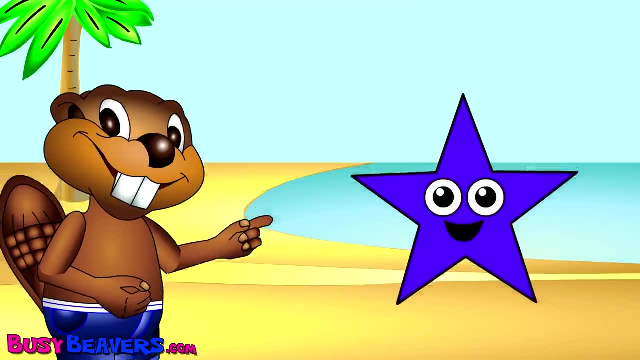 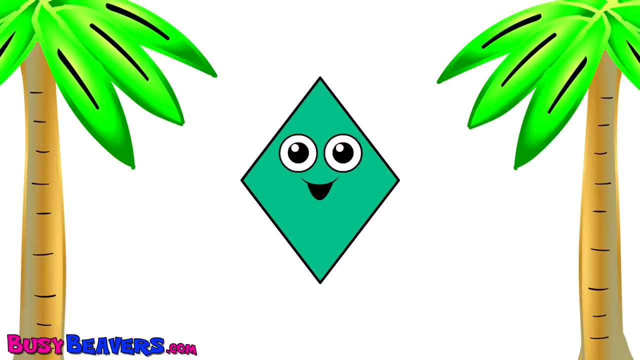 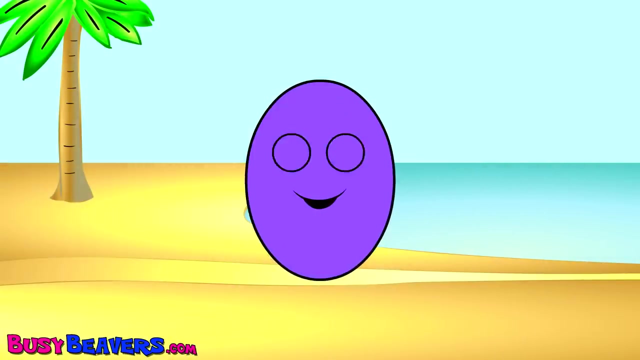 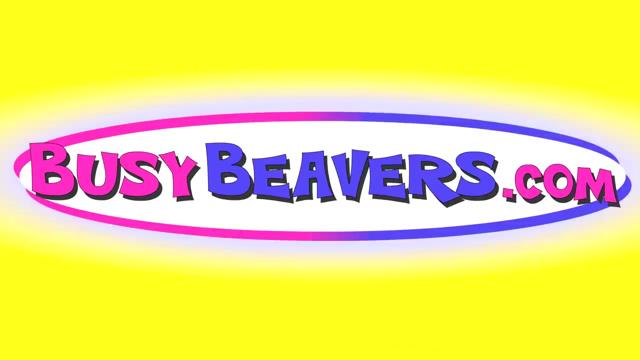 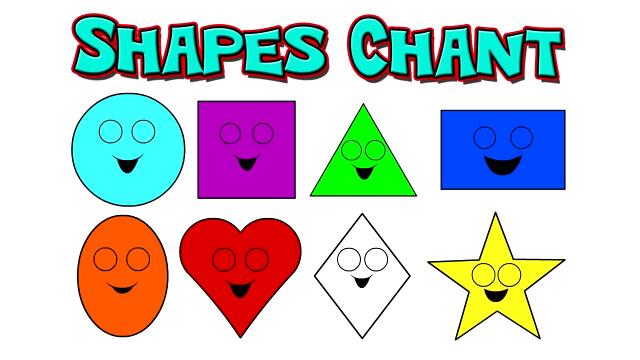 rectangle: Oval heart, diamond star. Oval oval heart heart, diamond, diamond star. Oval oval oval bell, bell, bell, bell. rainbow bell shapes Chants Circle Square. 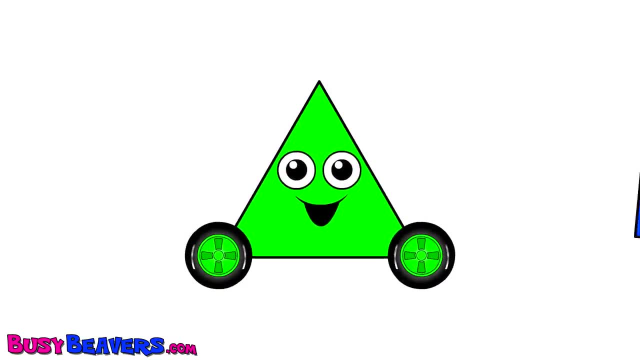 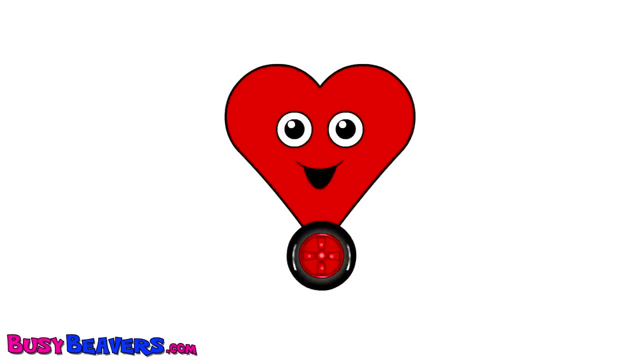 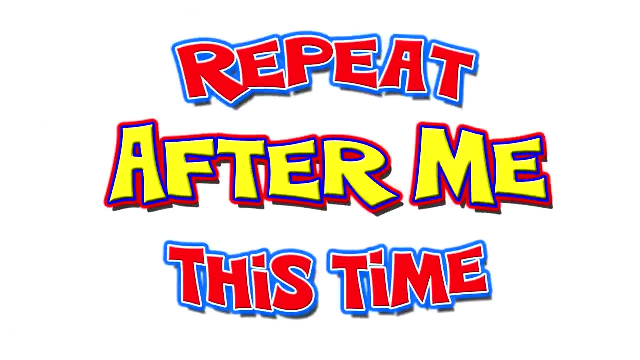 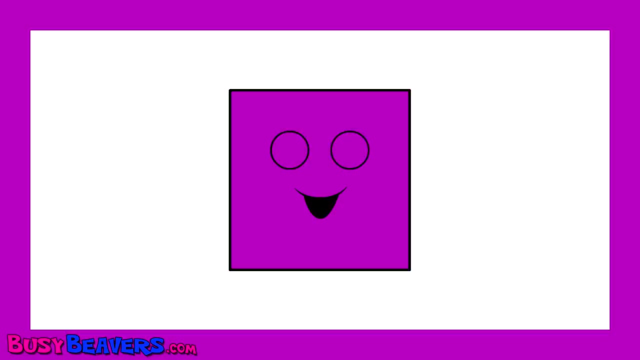 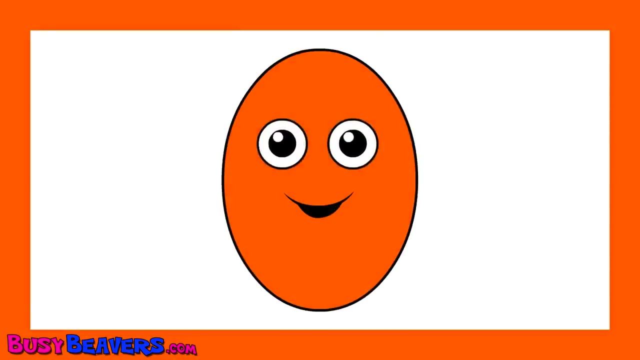 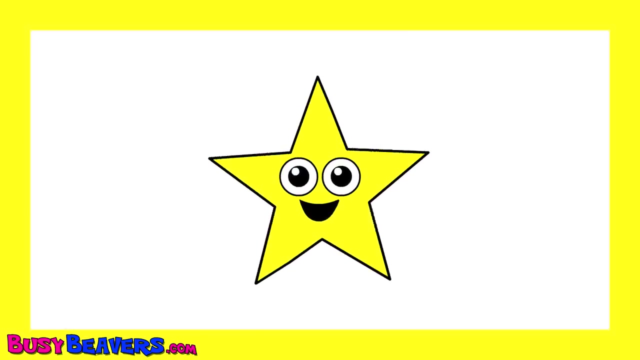 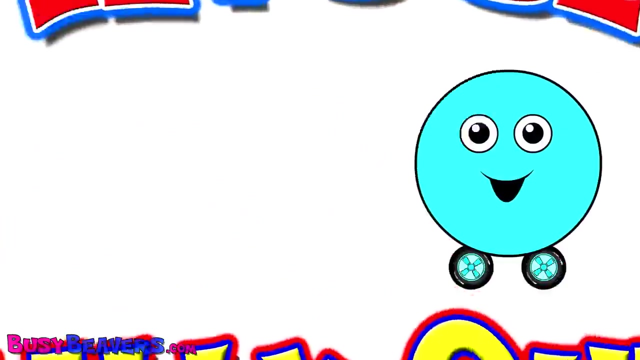 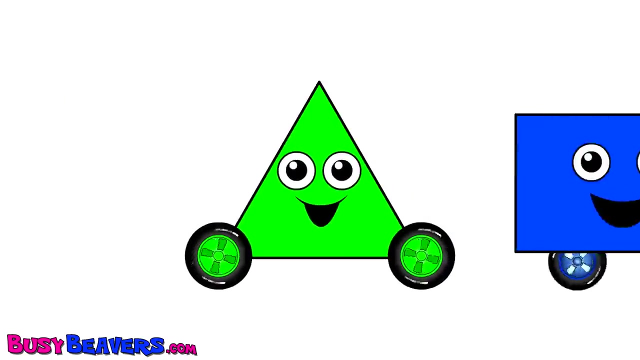 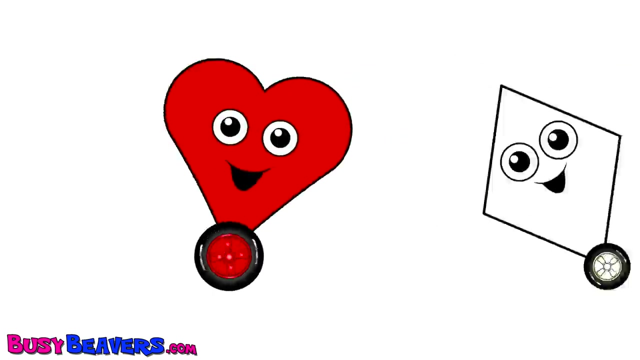 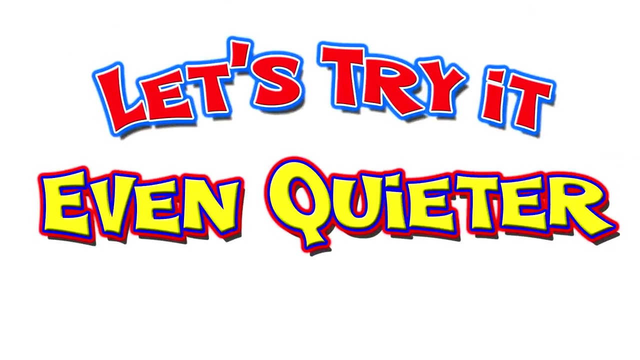 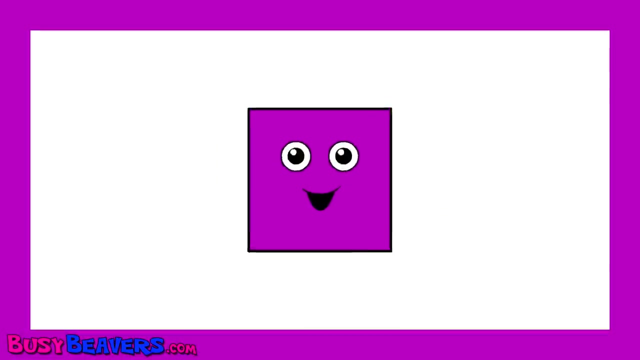 Circle, Circle, Triangle, Rectangle, Oval Heart, Diamond Star. Repeat after me this time: Circle Square, Triangle, Rectangle, Rectangle, Oval Heart, Diamond Star. Let's be really quiet this time. Circle Square, Triangle, Rectangle, Oval Heart, Diamond Star. Let's try it even quieter. Circle, Circle Square. 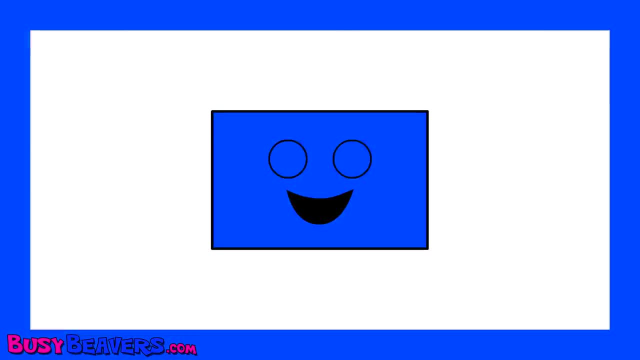 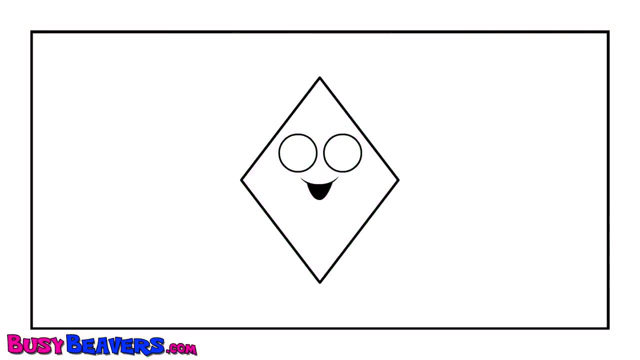 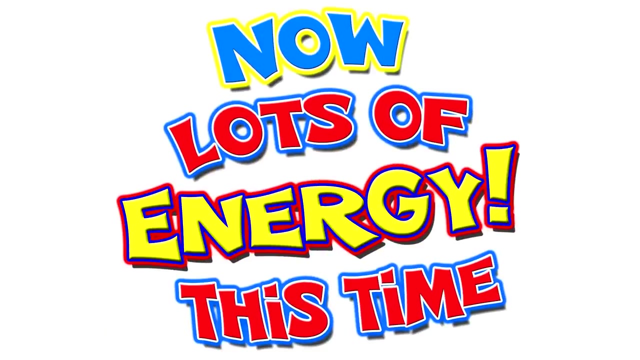 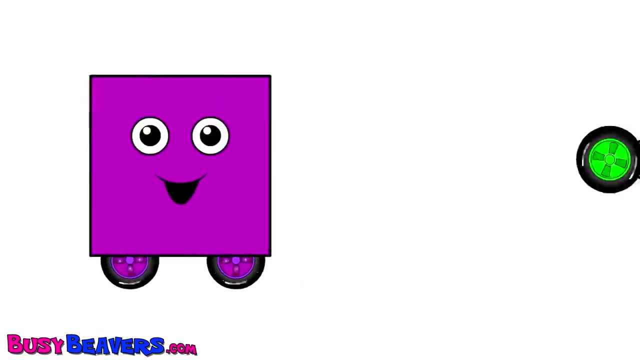 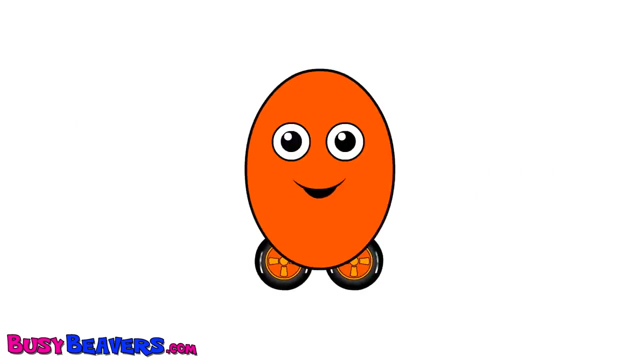 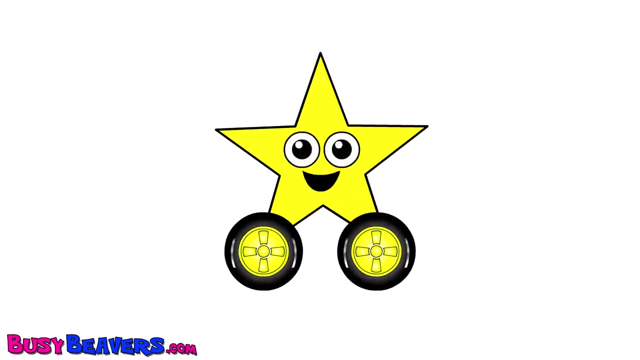 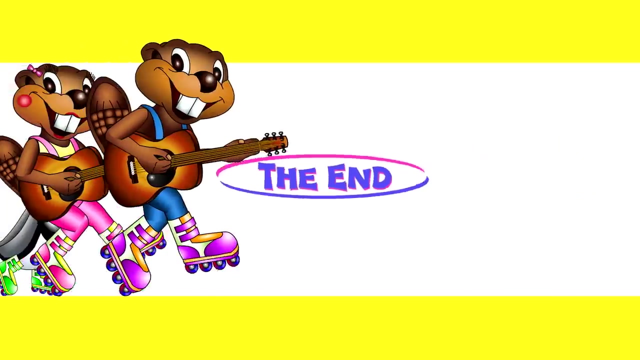 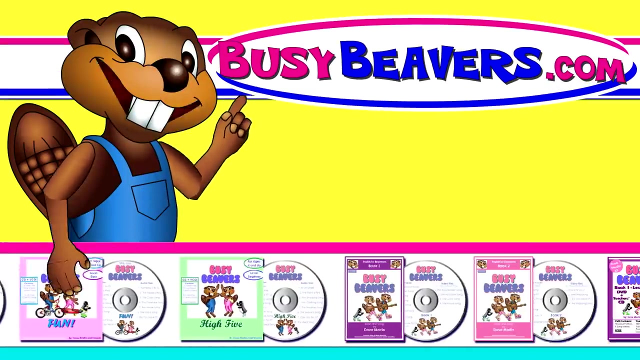 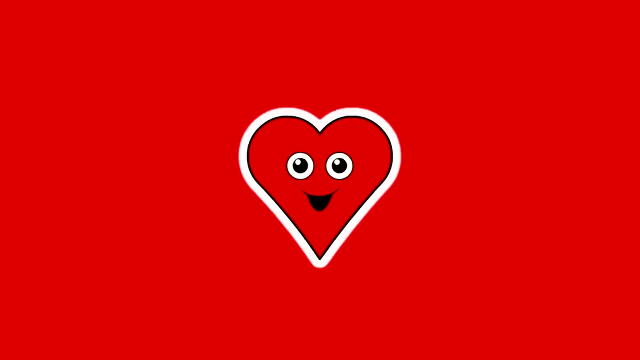 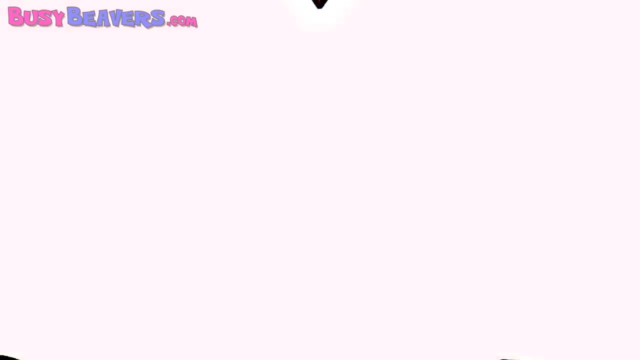 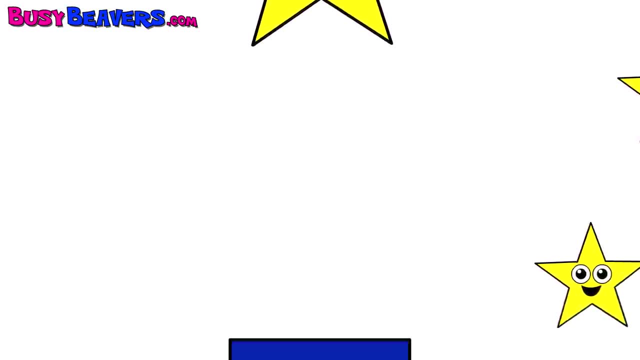 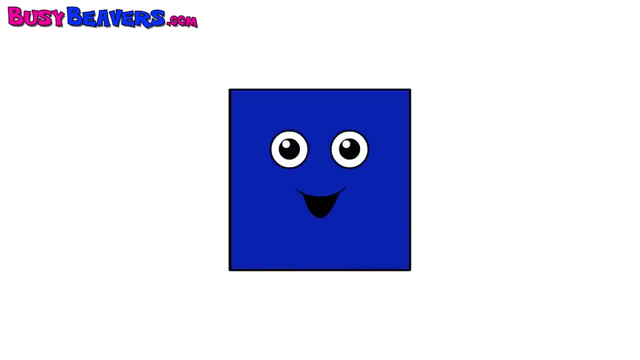 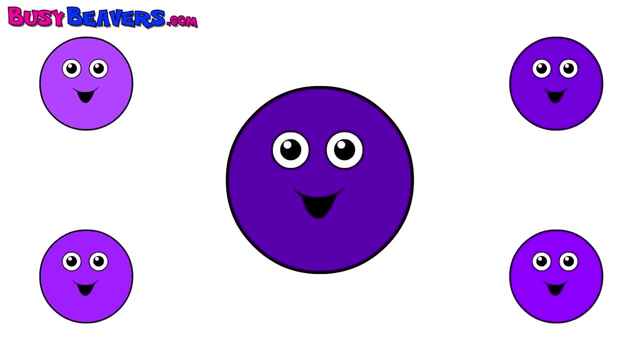 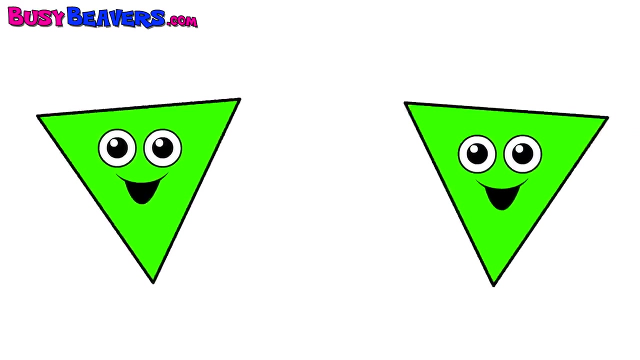 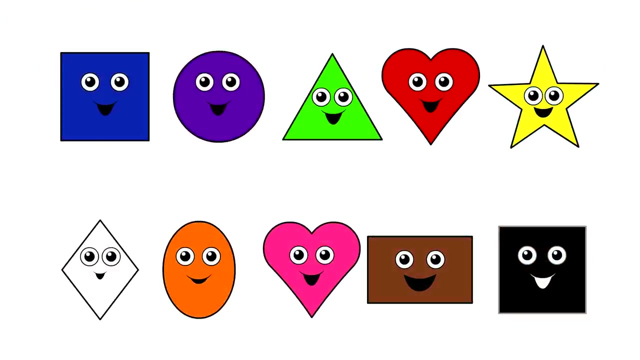 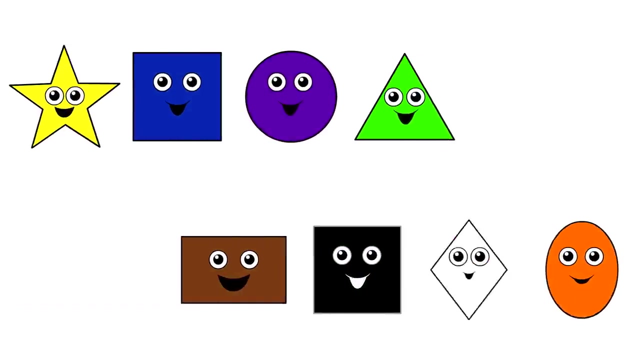 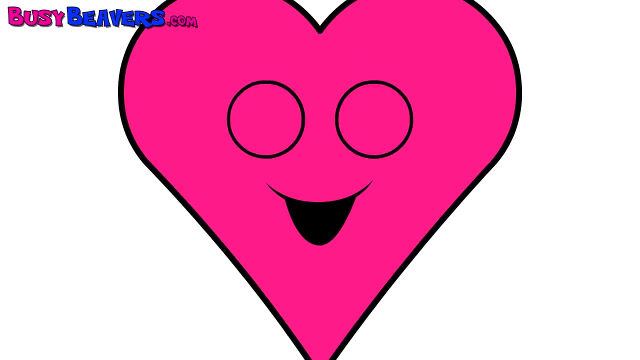 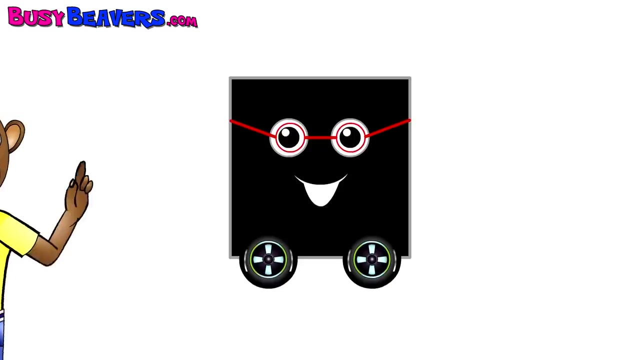 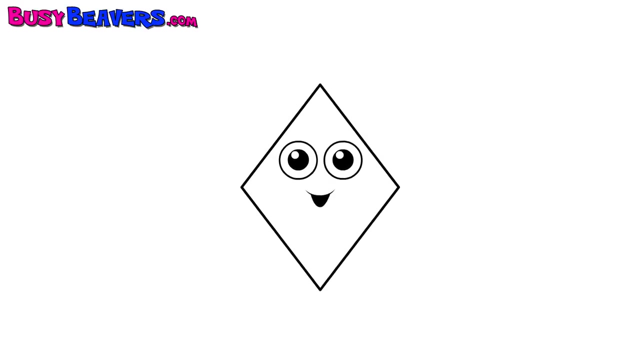 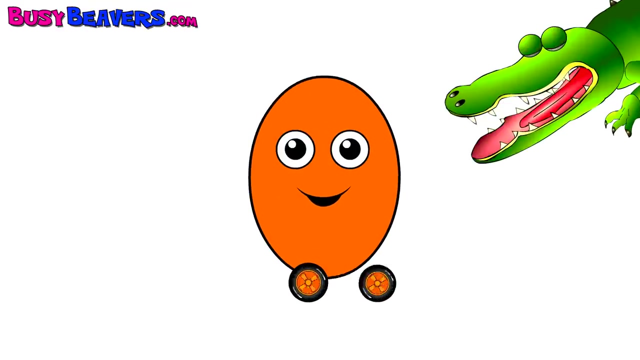 Yellow star, Blue square, Blue square. Purple circle- It's a purple circle, Purple circle. Green triangle, Green triangle. Pink heart, Pink heart. Black square- Hey, It's a black square, Black square. White diamond, White diamond. Orange oval: Oh, It's an orange oval, Orange oval. 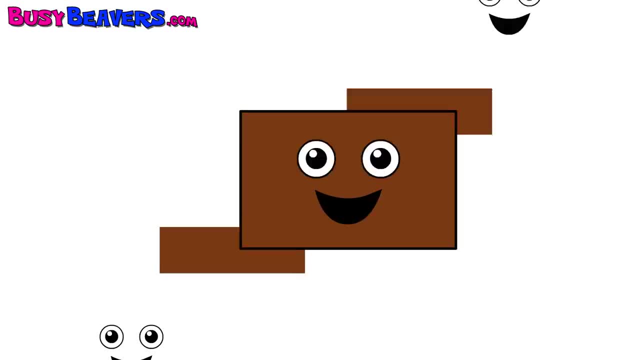 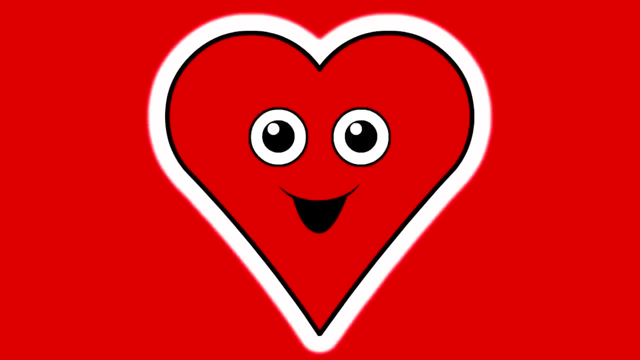 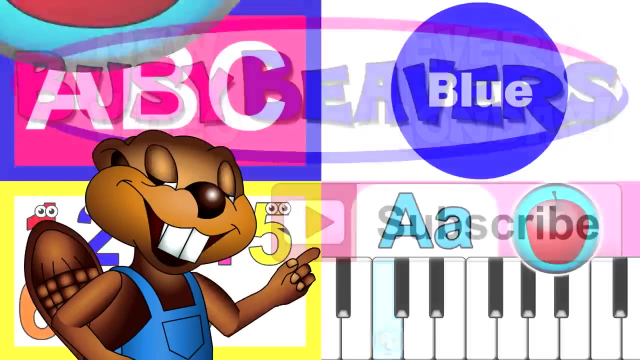 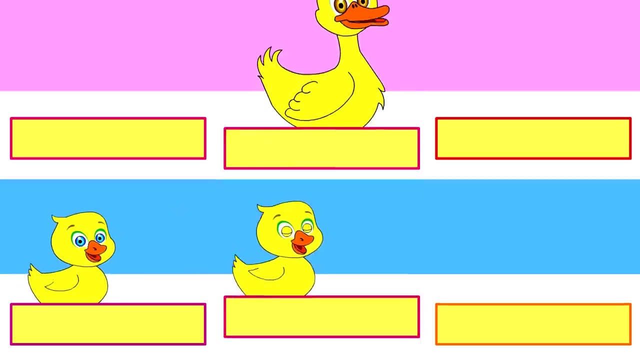 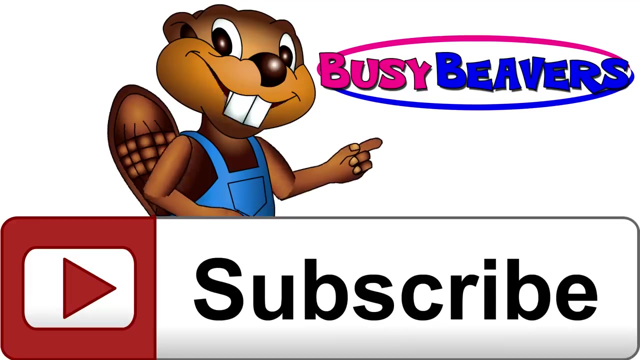 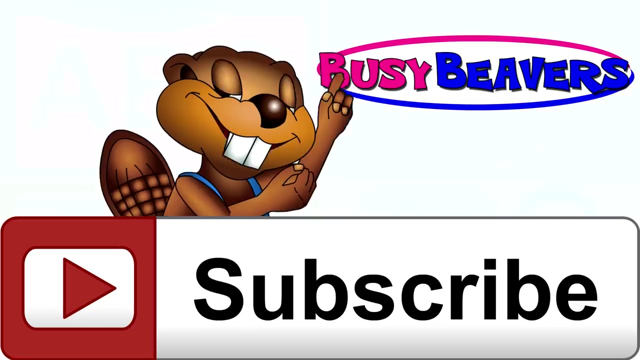 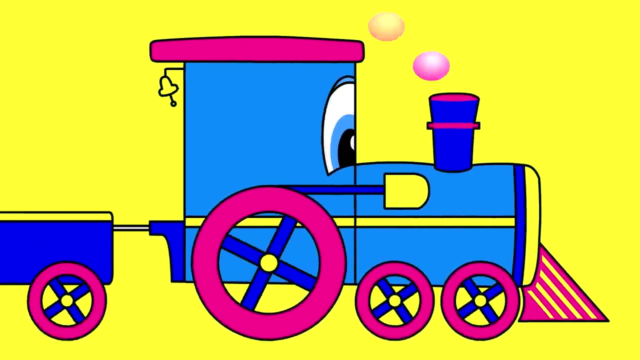 Brown rectangle, Brown rectangle, Green triangle, Global-Yon, GUI, Red-City, BlueBull, BlueM Hare, Peacock, White・・ Peacock, I love Peacock. Internet is the only place in the world where you can listen to music. Steamy Steamer, That's my name. 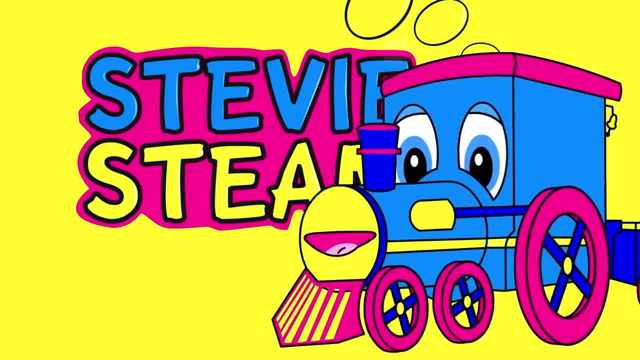 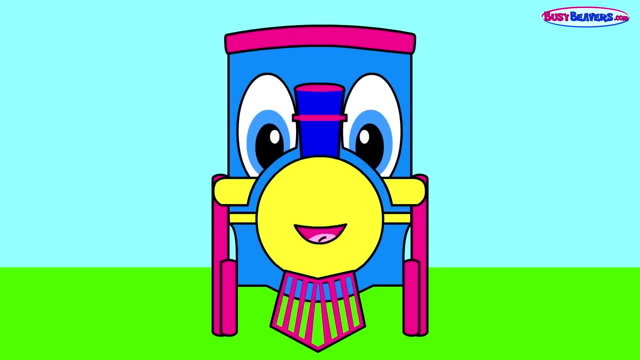 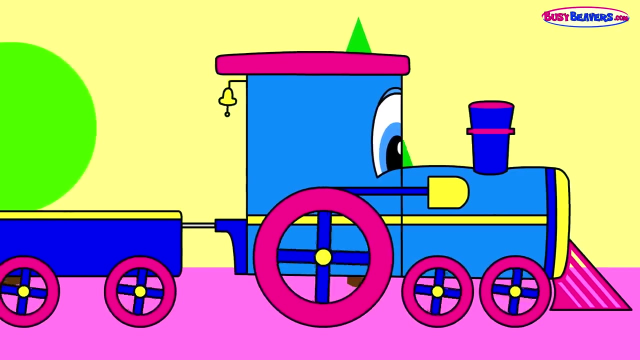 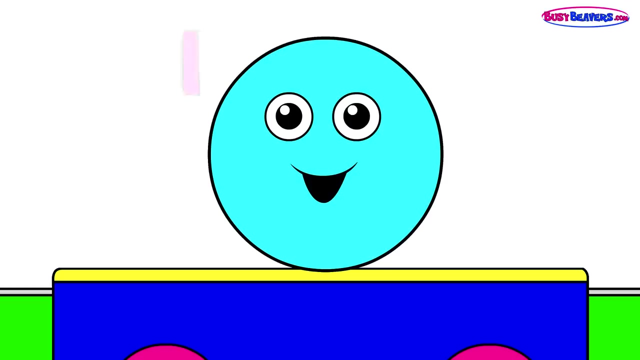 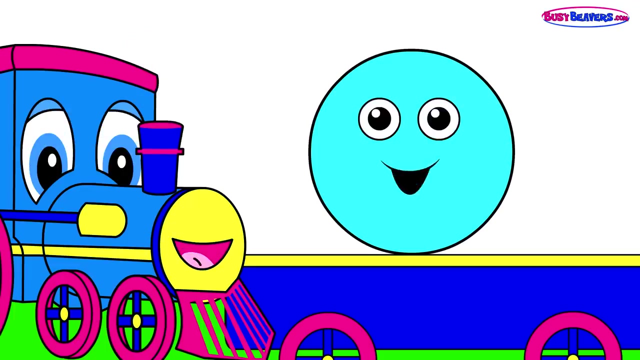 Steamy Steamer, I'm a train. Hello, I'm Steamy Steamer, I'm a train. Today I'm pulling some shapes. Let's go say hi to the shapes and count them. Circle One, One circle, Hello circle. Hello Steamer, Cool circle. 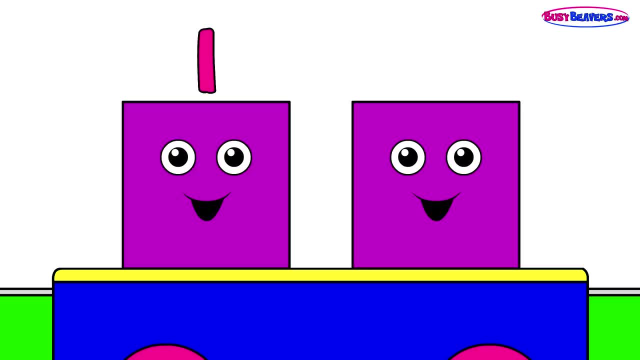 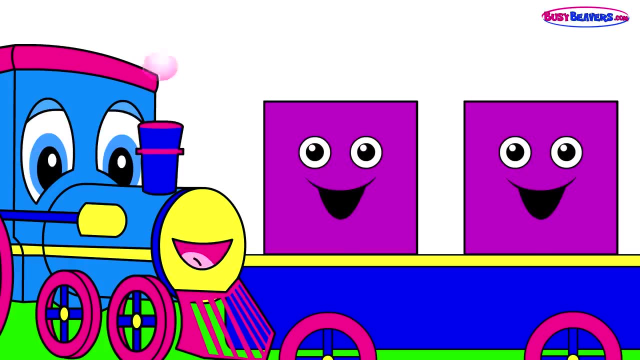 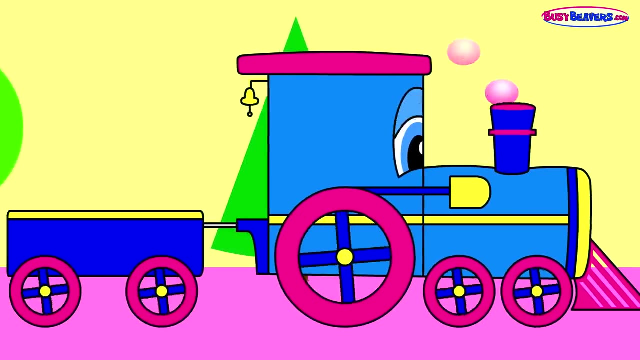 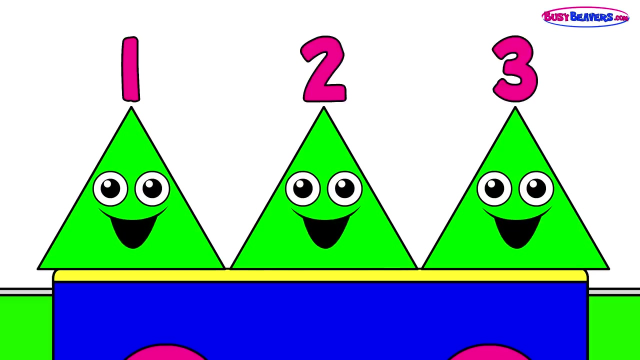 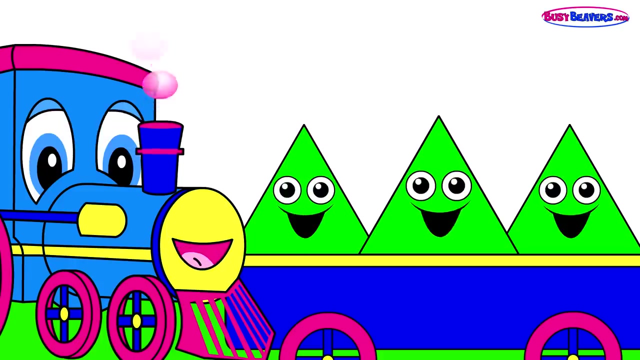 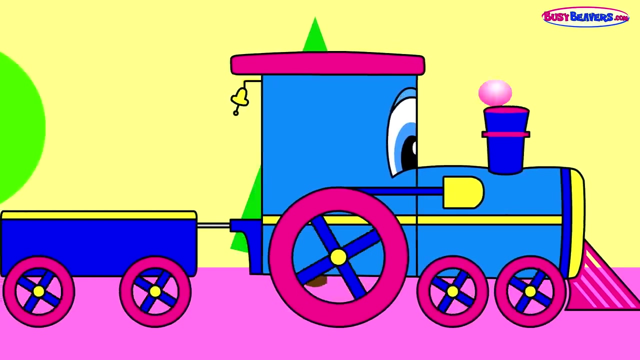 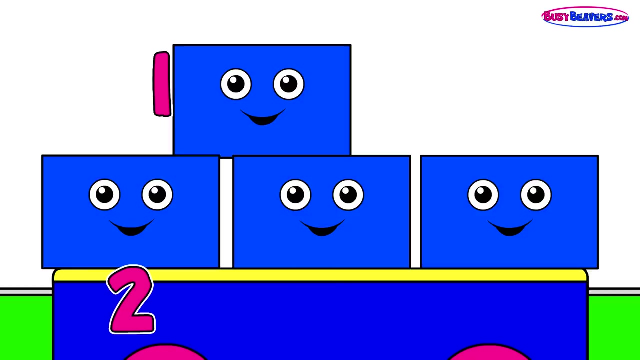 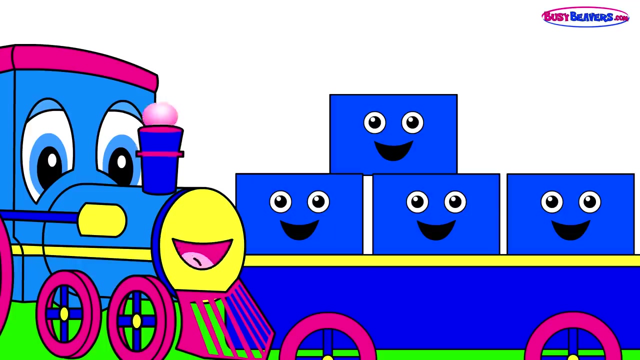 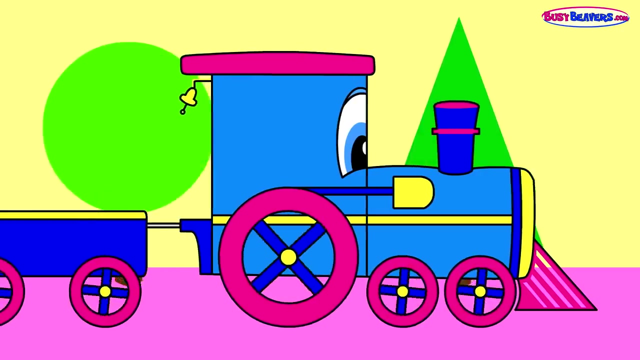 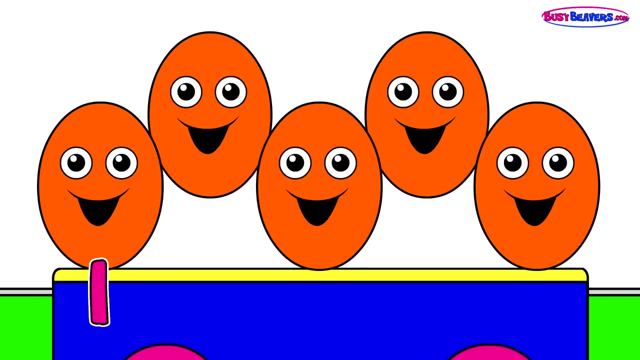 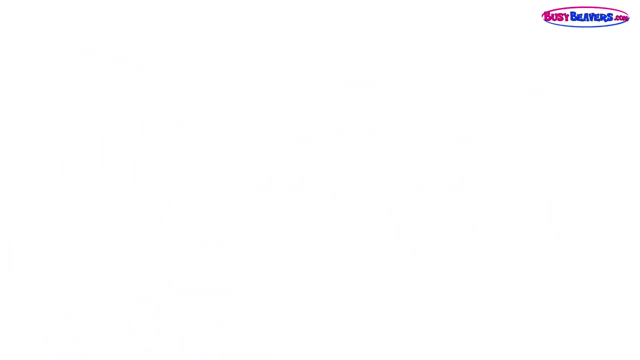 Square. One, Two, Two, squares, Hi, squares, Hi, Steamy Steamer, Square. Triangle One, Two, Three, Three. triangles, Hello, triangle, Triangle, Hello, Nice shapes. Rectangles One, Two, Three, Four, Four. rectangles, Hi, rectangles, Hi, Steamy Steamer, Love the rectangles. Ovals. one, two, three, four, five, five, ovals, hey, ovals, hi, how you doing. well that's. 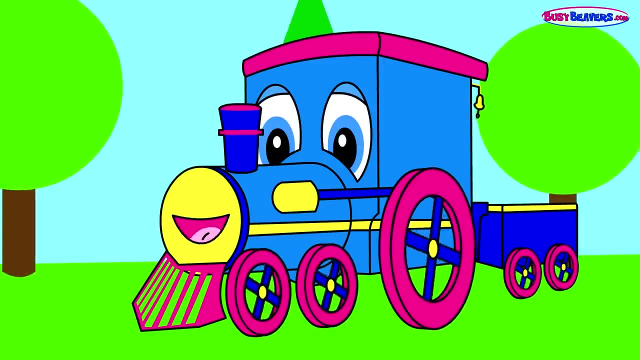 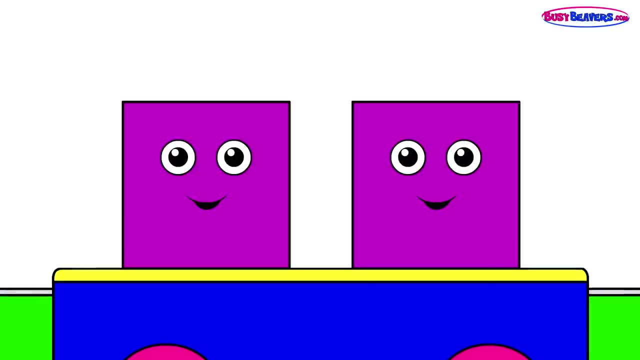 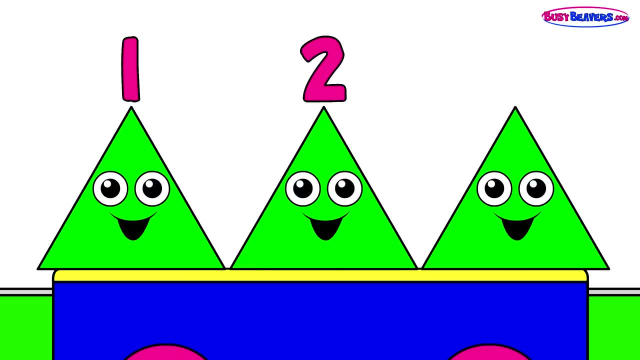 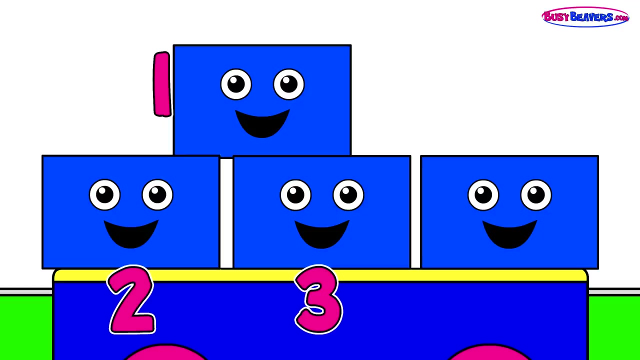 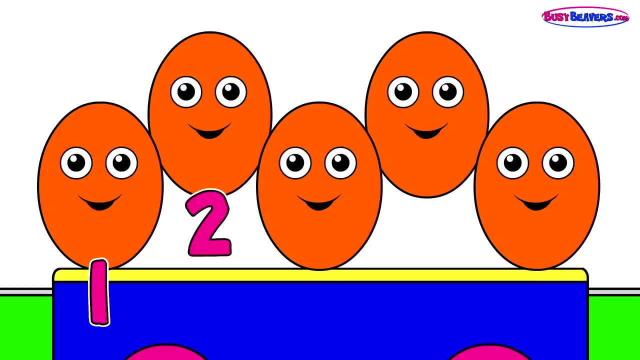 all the shapes for today. let's count them one more time: one circle: one two squares one, two, three. triangles: one, two, three, four rectangles: one, two, three, four rectangles one, two, three, four, five ovals. all aboard, here we go. 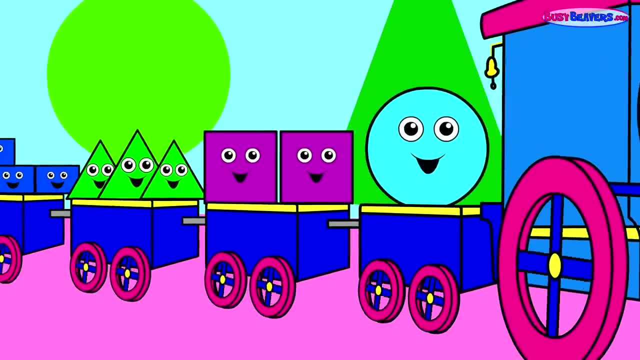 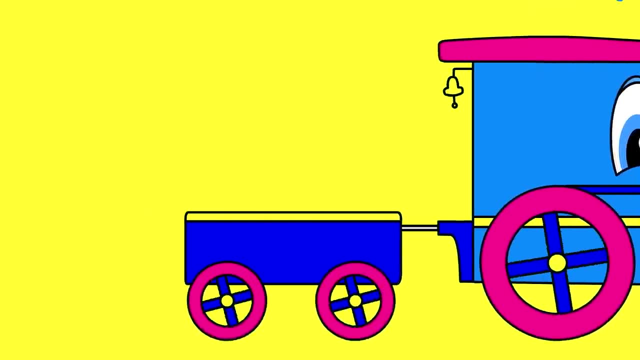 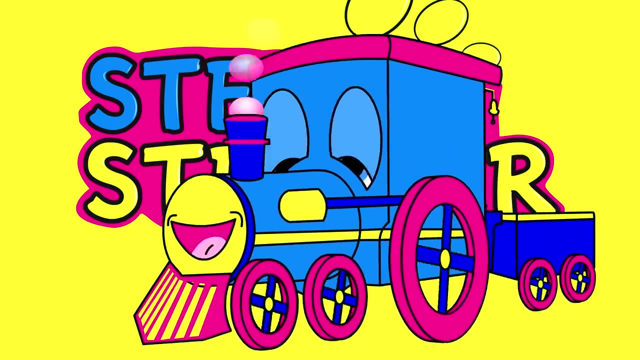 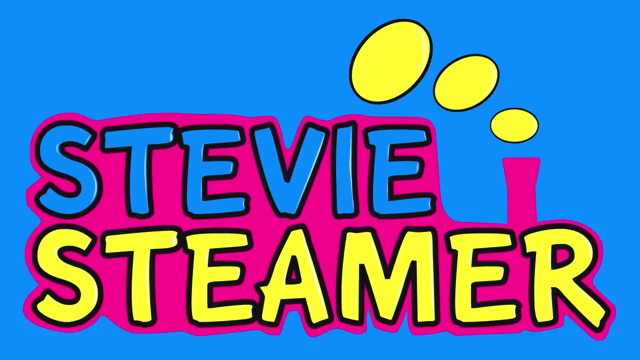 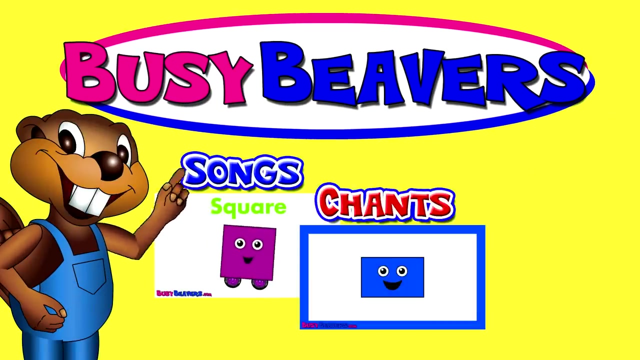 steamy steamer, that's my name. steamy steamer. steamy steamer, that's my name. steamy steamer, I'm a train. Welcome to the Busy Beavers collection of shapes, songs, chants and lessons. 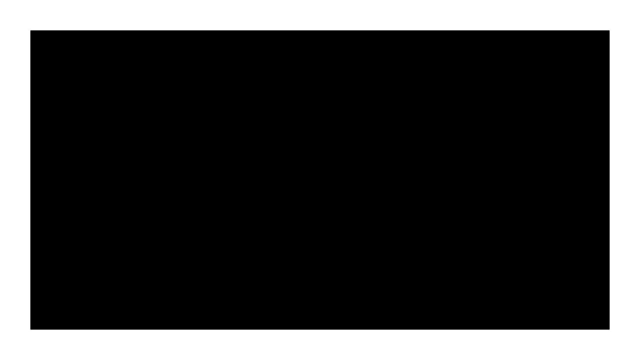 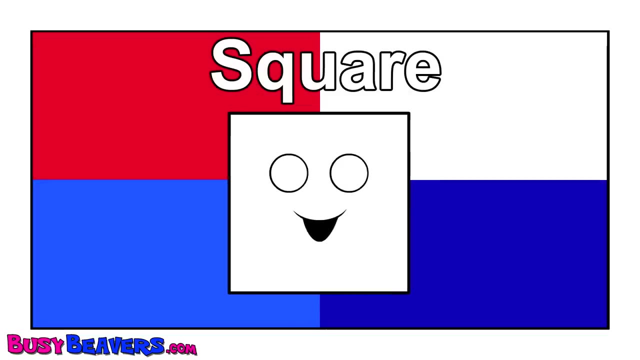 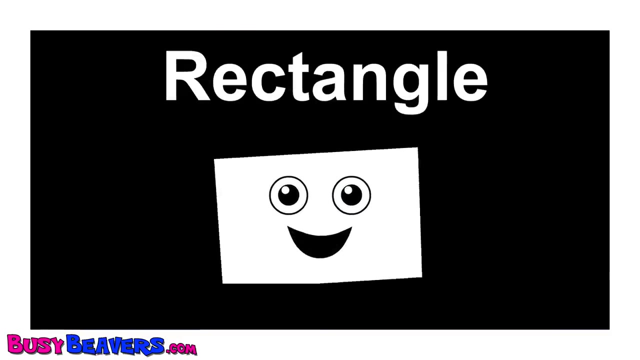 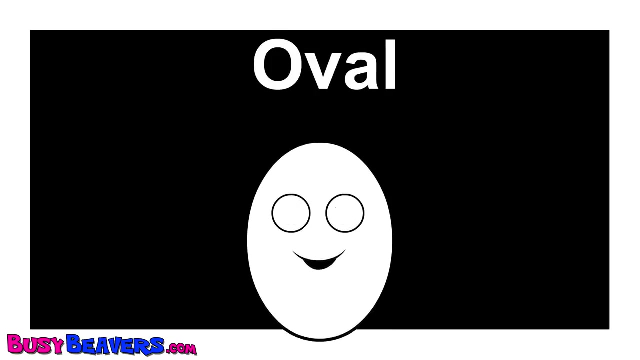 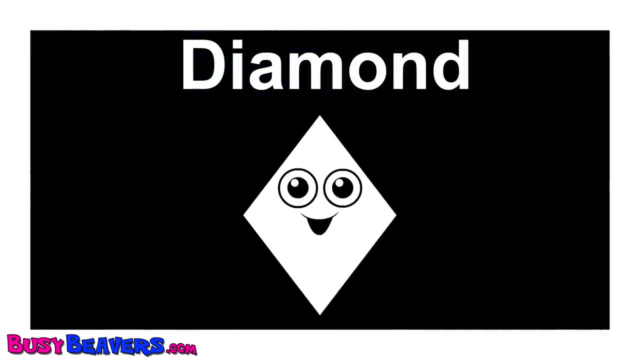 Nashville Shapes, Hoedown Circle, circle, circle, circle, Square, square, square, square, Triangle, triangle, triangle, triangle, Rectangle, rectangle, rectangle, rectangle, Oval, oval, oval, oval, Heart, heart, heart, heart, Diamond, diamond, diamond, diamond. 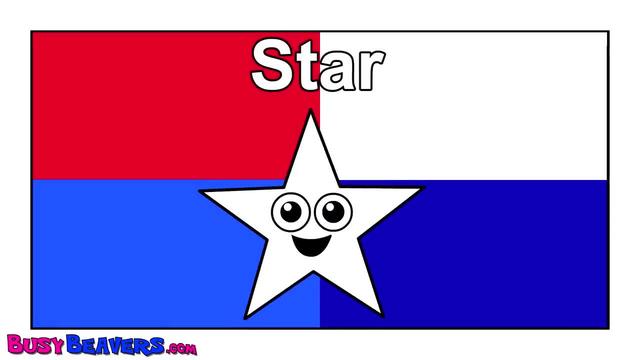 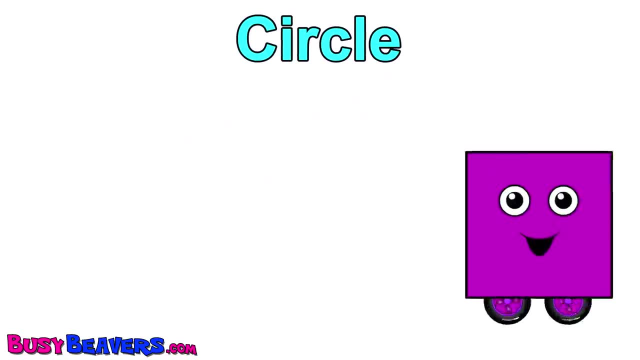 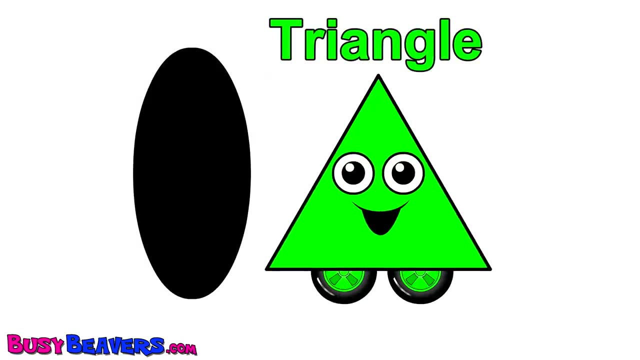 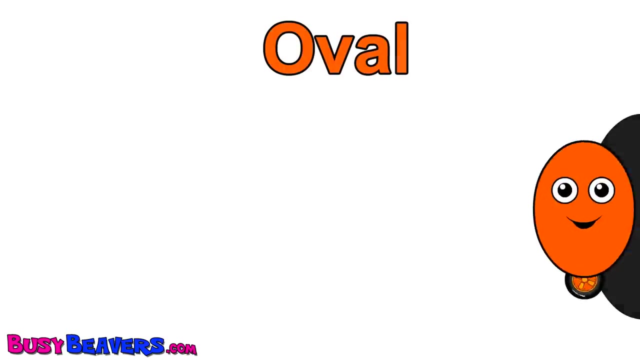 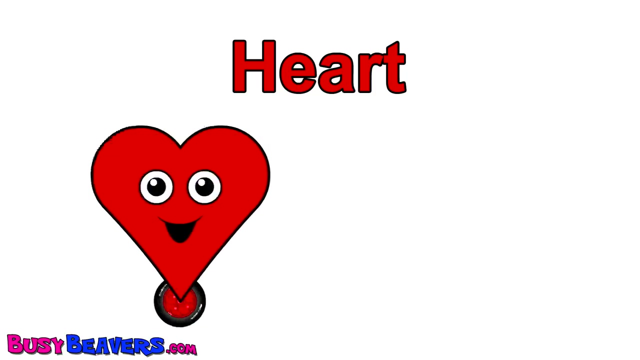 Star star, star Circle, circle, circle, circle, Square, square, square, square, Triangle, triangle, triangle, triangle, Rectangle, rectangle, rectangle, rectangle, Oval, oval, oval, oval, Heart, heart, heart, heart, Diamond, diamond, diamond, diamond. 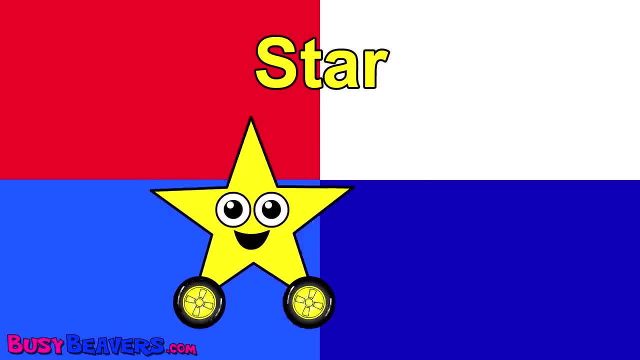 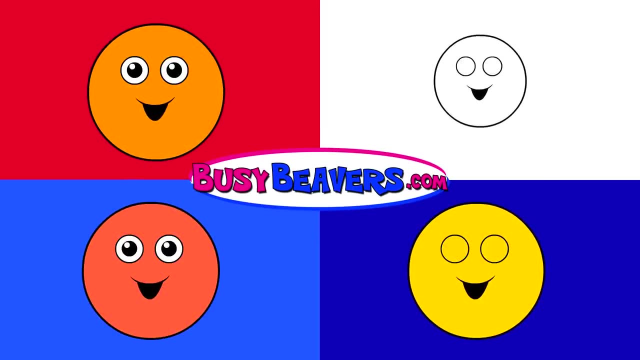 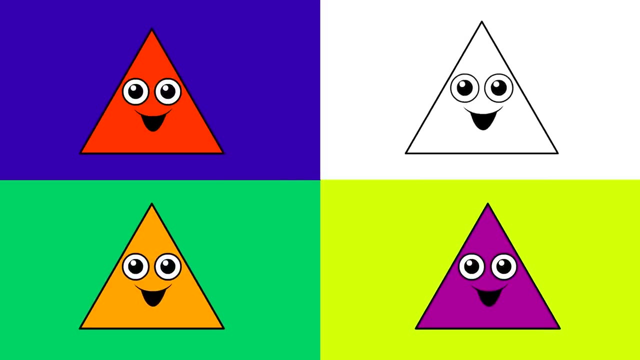 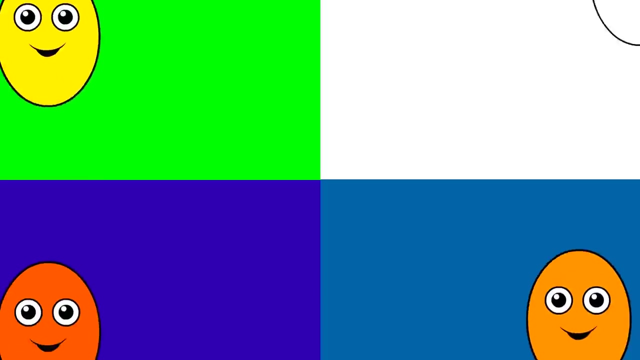 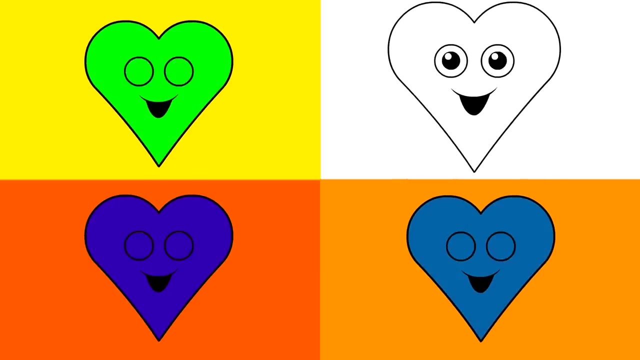 Star star, star Circle, circle, circle, circle, Square, square, square, square, Triangle, triangle, triangle, triangle, Rectangle, rectangle, rectangle, rectangle, Oval, oval, oval, oval, Heart, heart, heart, heart, Diamond, diamond, diamond, diamond. 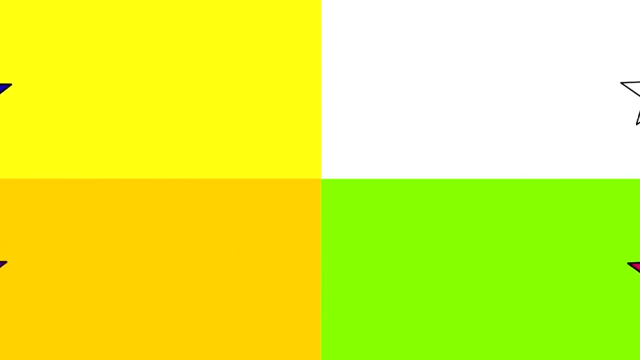 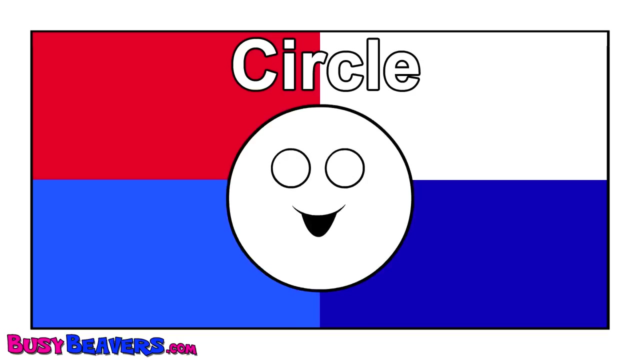 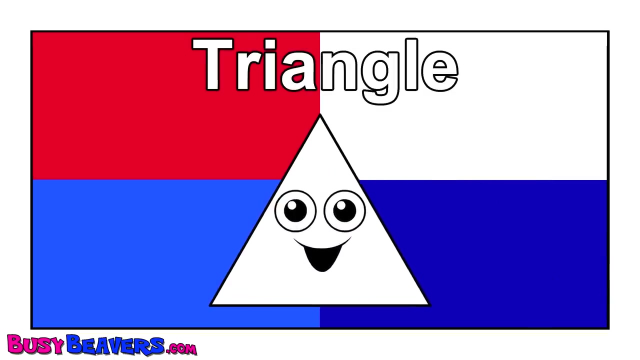 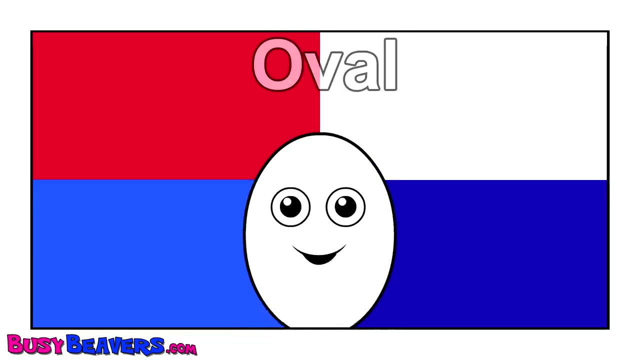 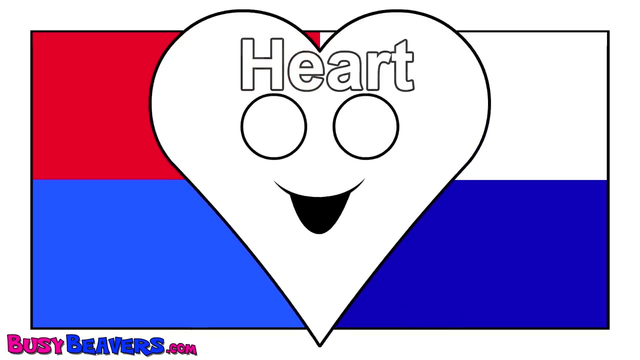 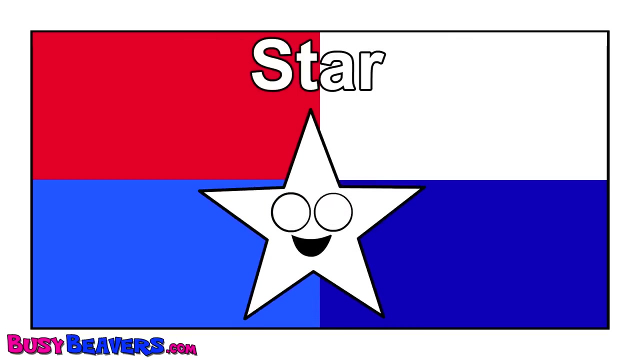 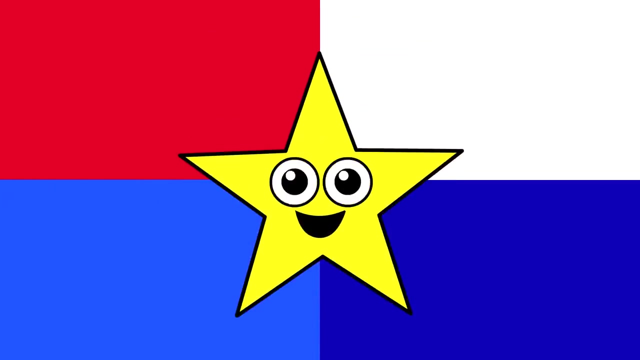 Star star, star Triangle, top, bottom Time time. when you're swinging, Point a finger at the sky. Who you want to be, We don't know. Aah, who I want to be. Who I want to be, Who I want to be, Skip Ad. 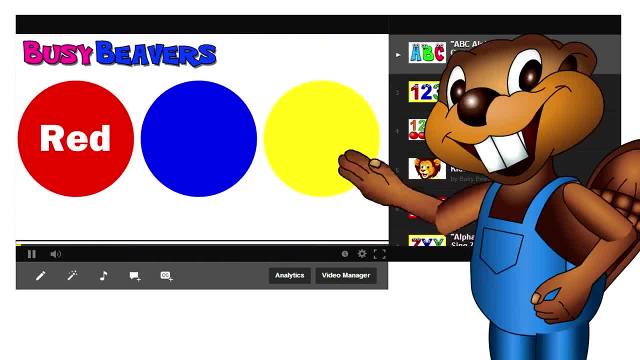 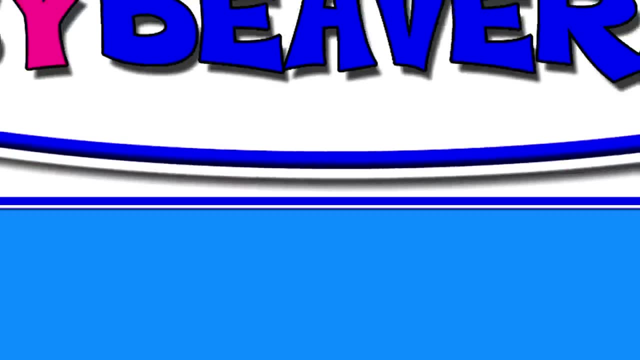 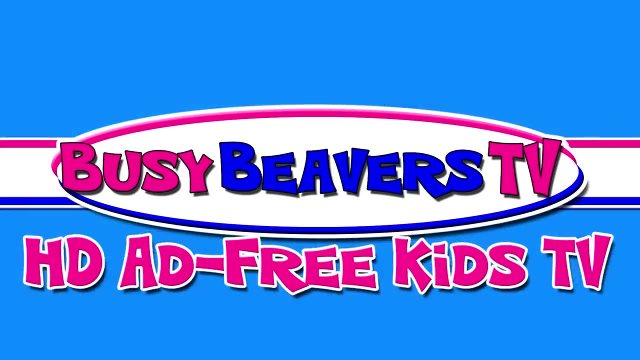 Skip Ad. Are you tired of watching ads before every video on YouTube? Oh, they're very frustrating. Hehe, I know Well. Busy Beavers have a new channel, Busy Beavers TV, where all of our kids' learning videos are in HD and ad-free. 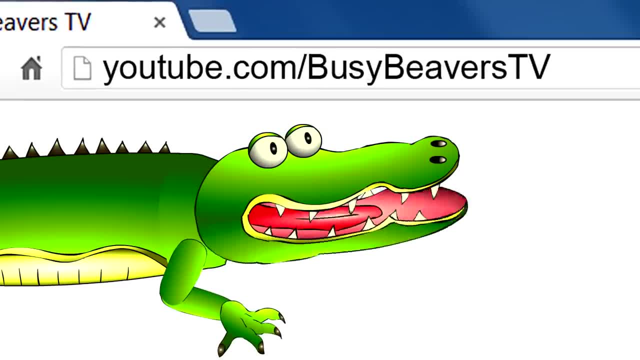 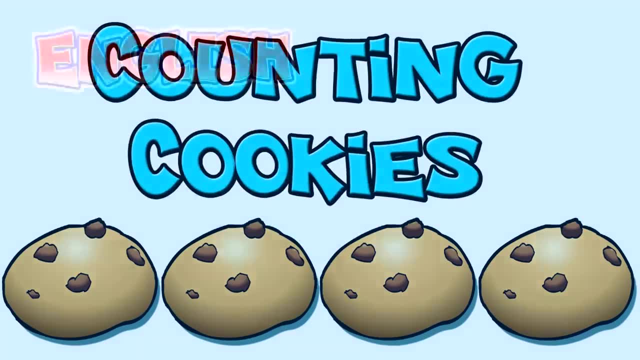 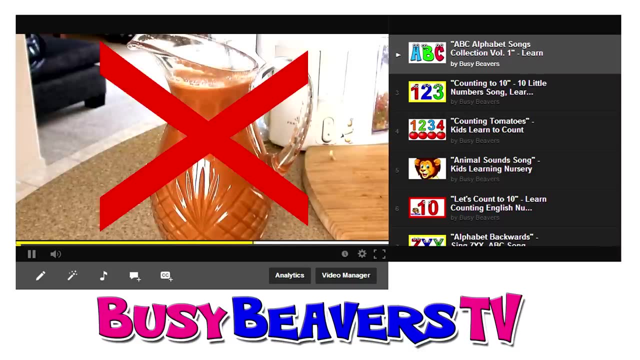 So let me get this straight: YouTubecom slash Busy Beavers TV has all of the Busy Beavers song videos and all of the kindy lesson videos, and I can learn to speak English, Chinese, Korean, Spanish and more, And there's no ads, no pop-ups and no commercials. 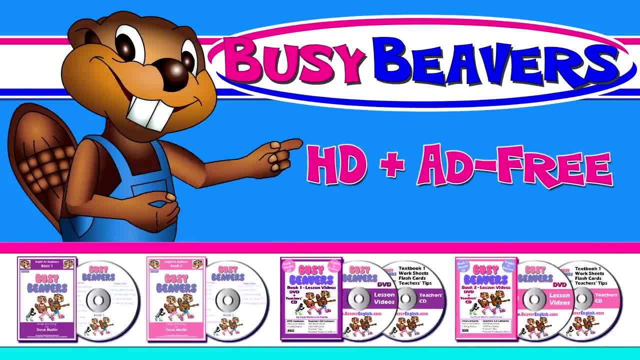 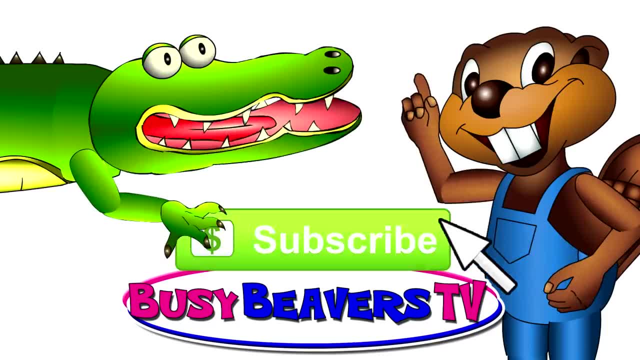 All of the great content from our free channel in HD and ad-free. That's it. I'm clicking that button and I'm not kidding. Do it. YouTubecom slash Busy Beavers TV for kids' learning videos in HD and ad-free. 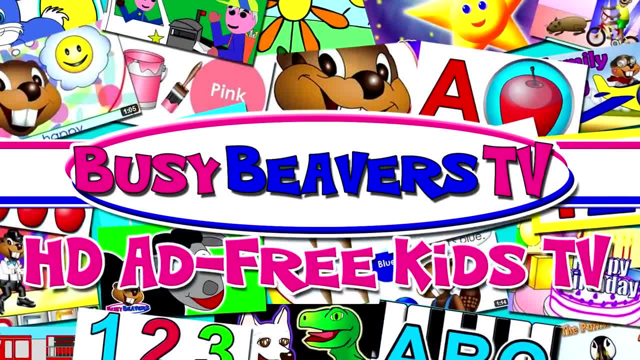 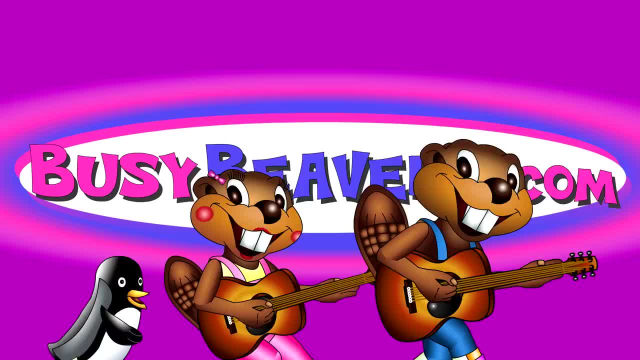 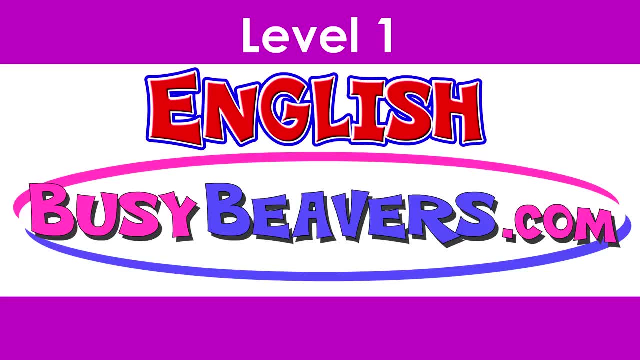 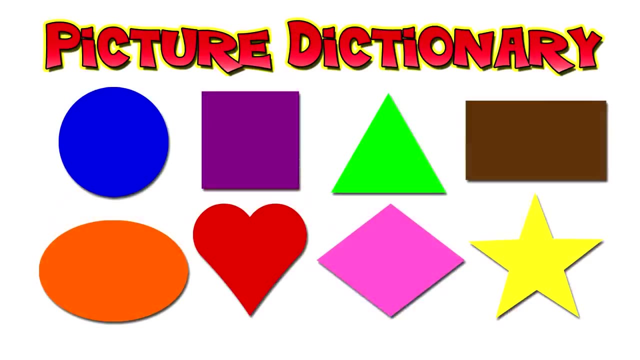 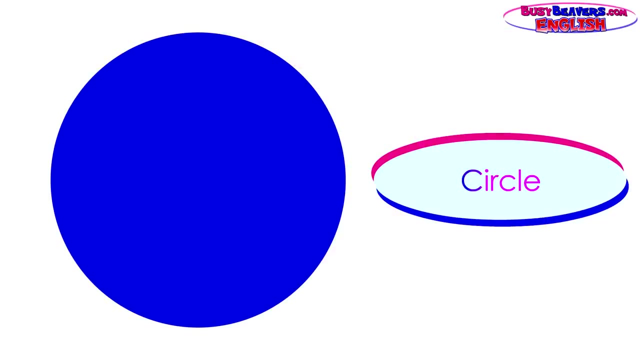 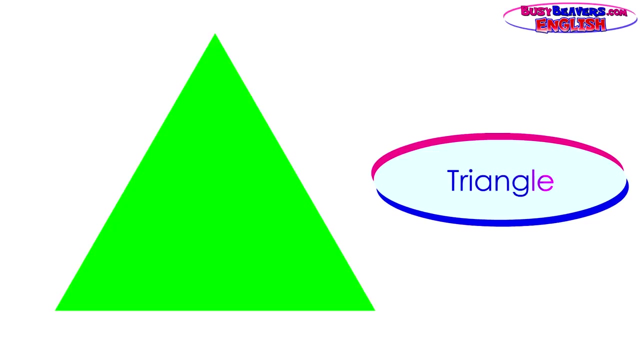 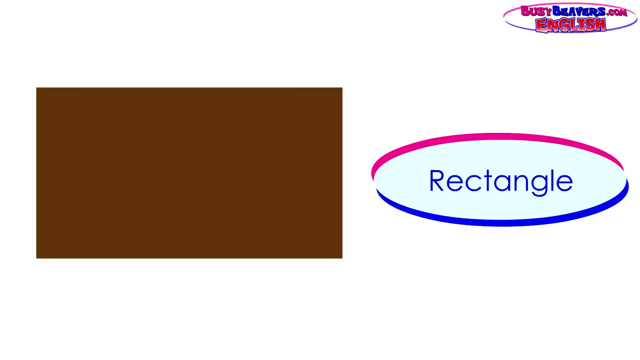 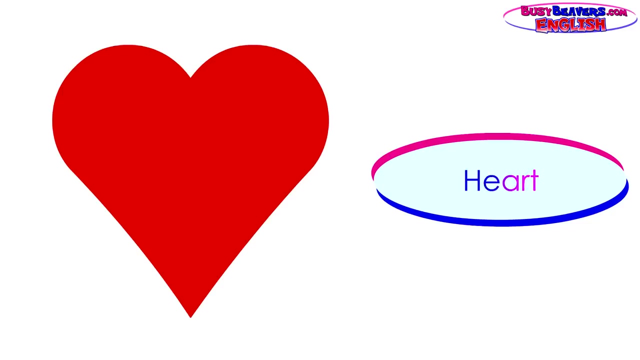 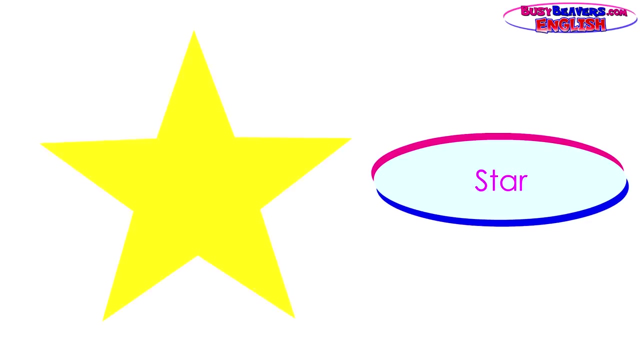 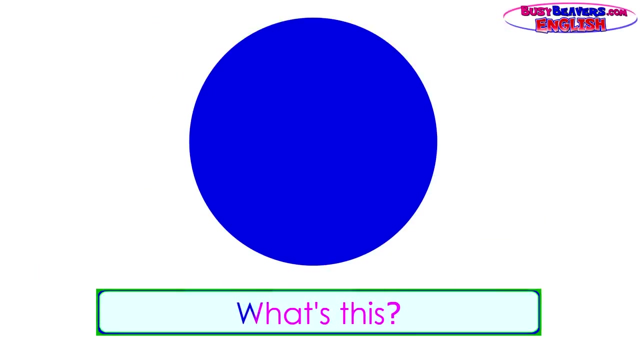 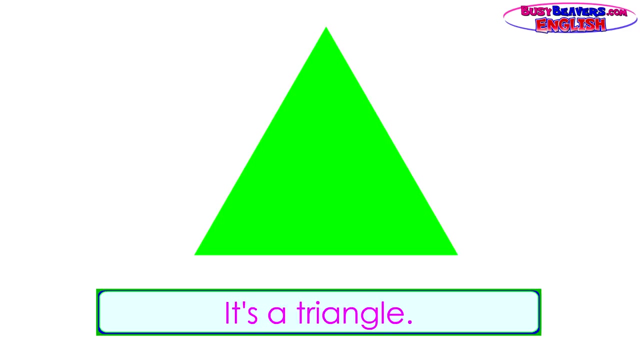 And ad-free Shapes: Lesson Circle, Square, Triangle, Rectangle, Oval, Heart, Heart, Heart, Diamond, Diamond, Diamond, Star, Star. What's this? It's a circle. What's this? It's a square. What's this? It's a triangle? It's a rectangle. 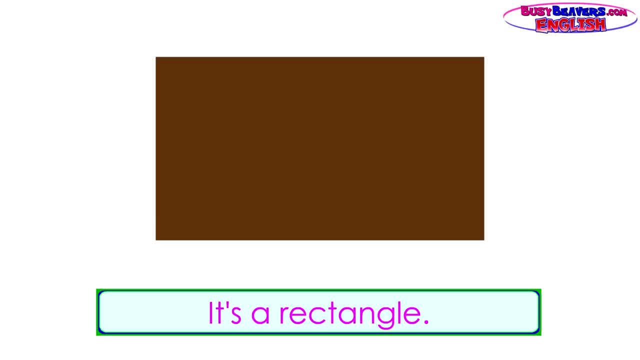 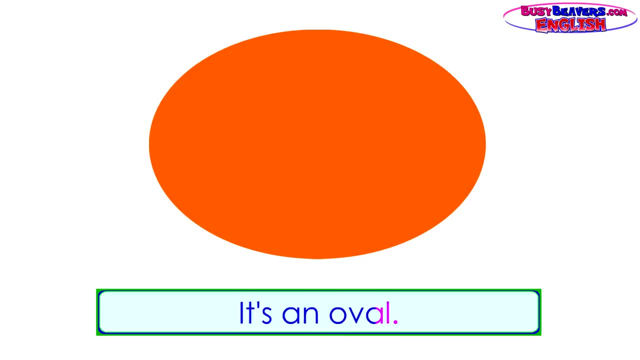 What's this? It's a rectangle. What's this? It's a rectangle. What's this? It's an oval. What's this? It's an oval. What's this? It's an oval. What's this? It's a heart. 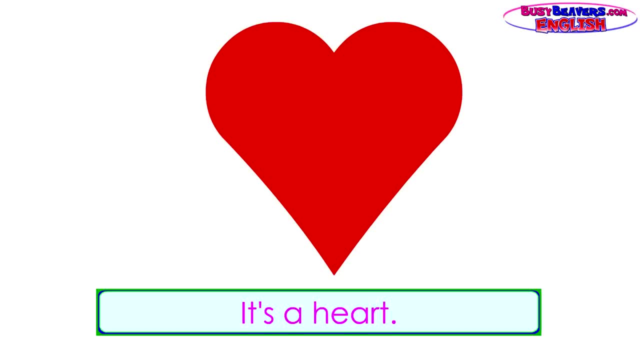 What's this? It's a heart. What's this, It's a heart. What's this? What's this? It's a diamond. What's this: It's a diamond. What's this? What's this? It's a star. 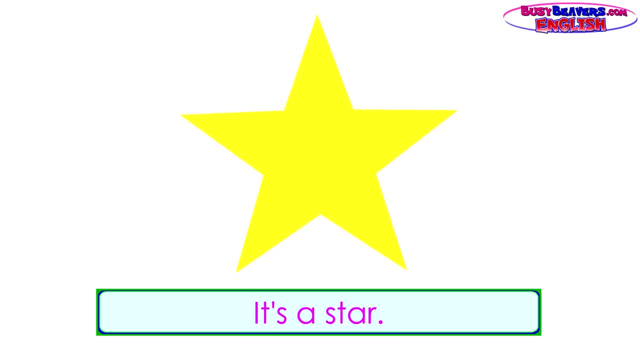 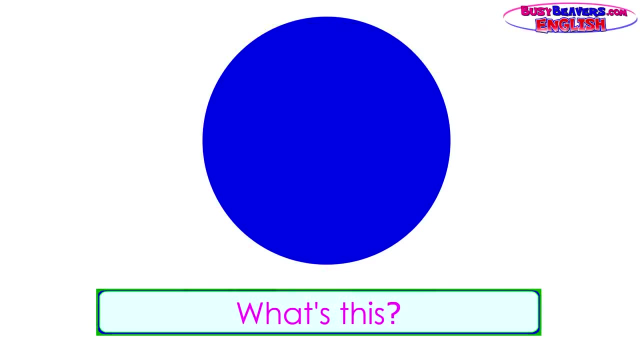 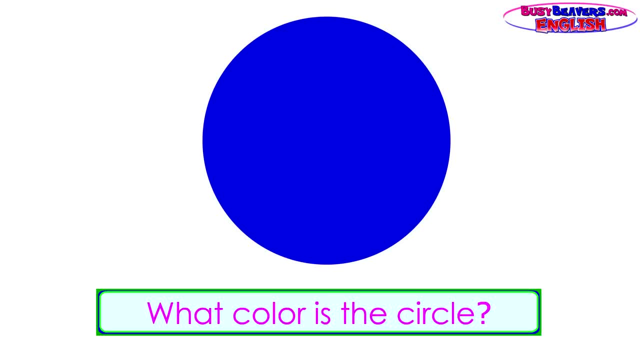 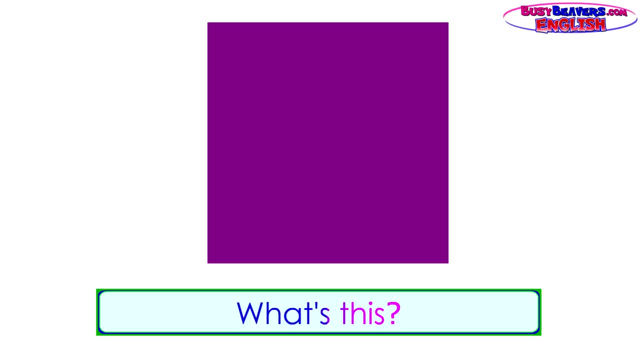 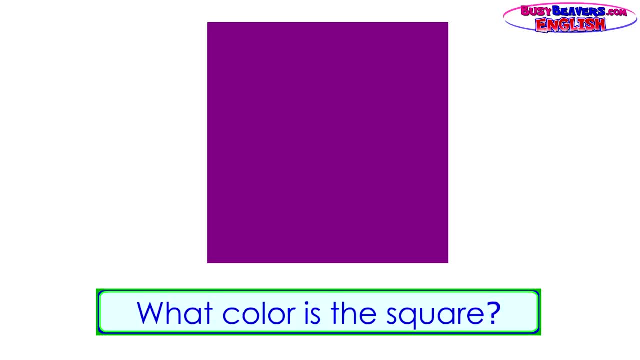 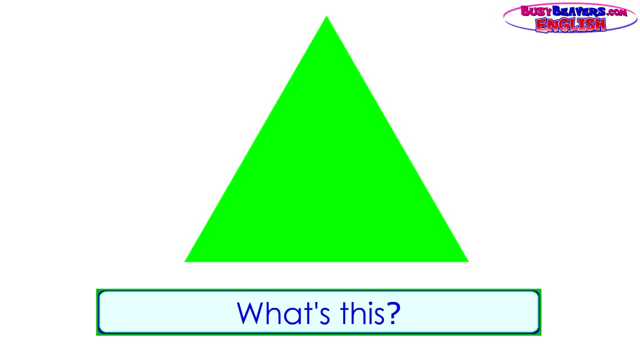 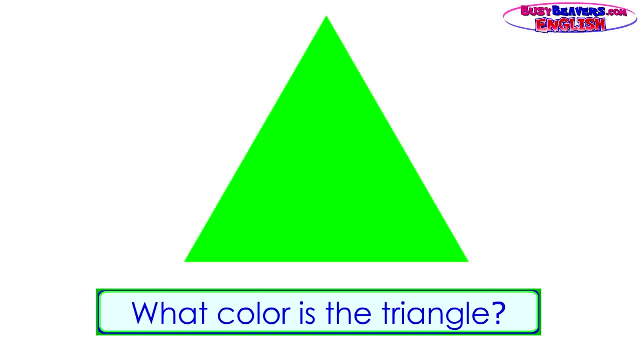 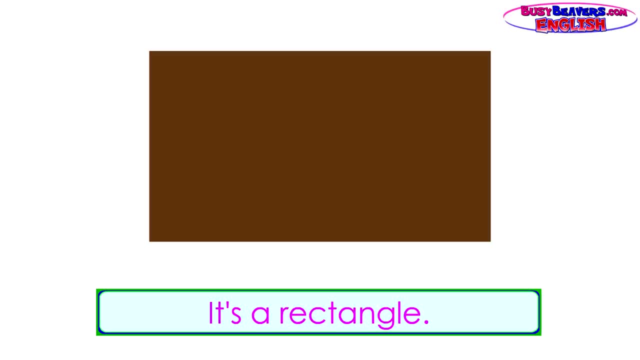 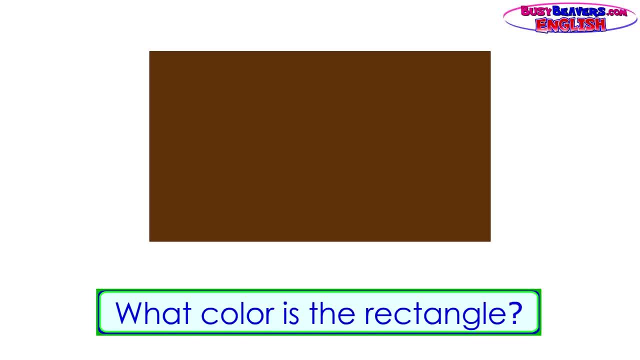 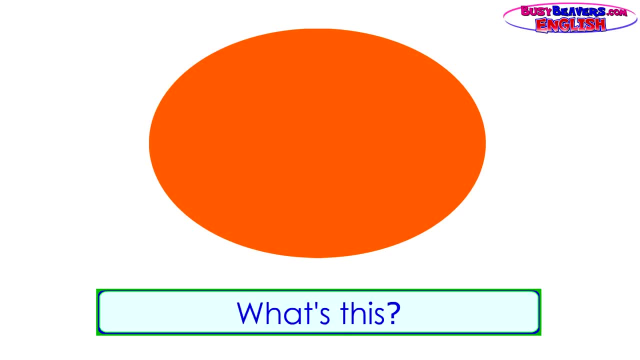 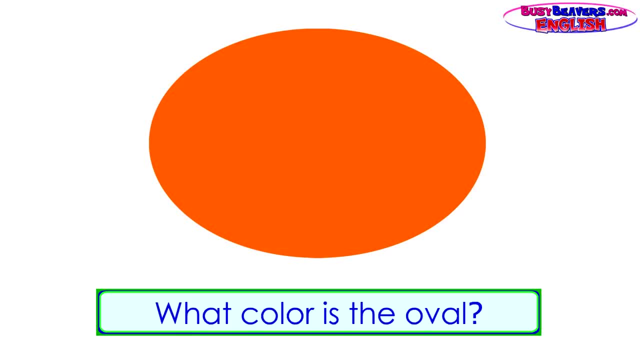 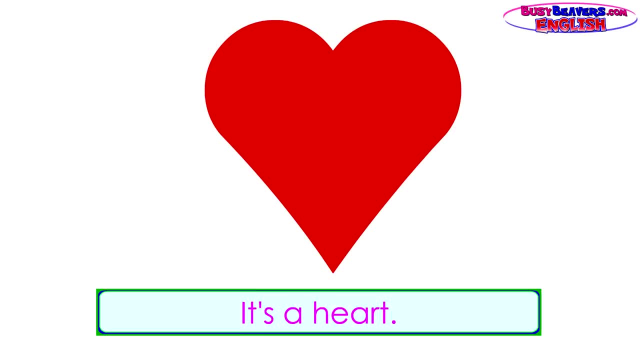 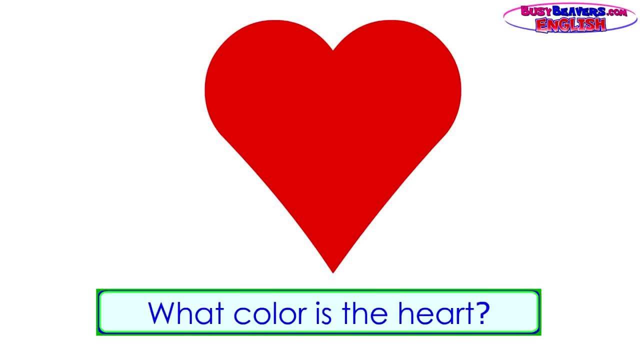 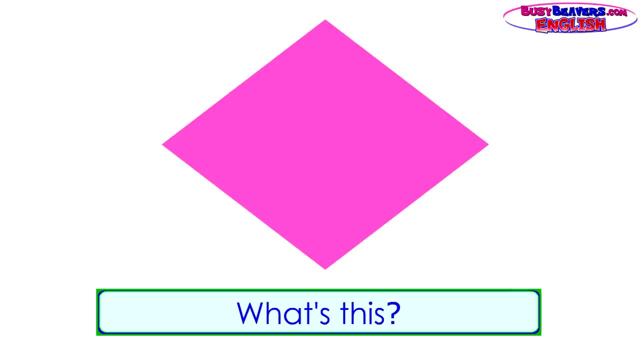 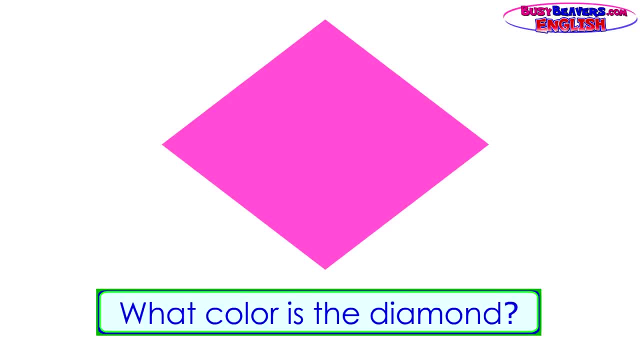 What's this? It's a diamond. What's this? It's a diamond. What's this? It's a diamond. What's this? What's this? It's a star. What color is the star? The star is yellow. 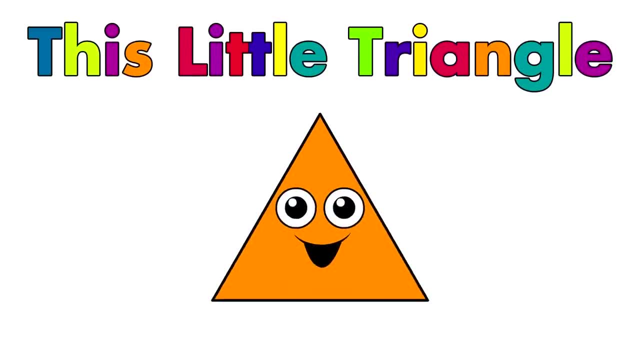 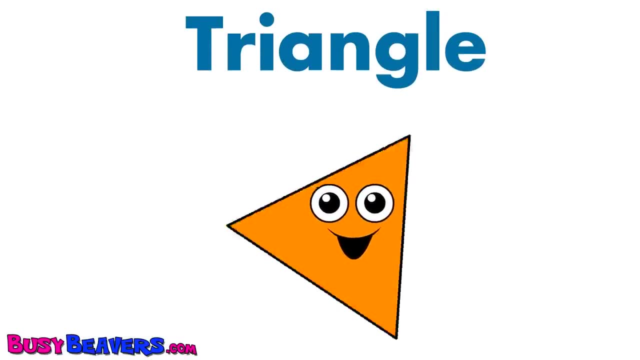 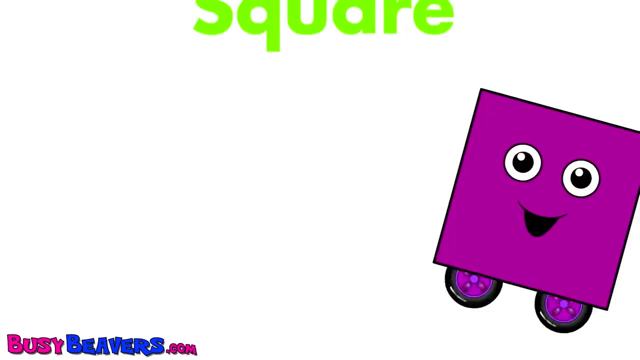 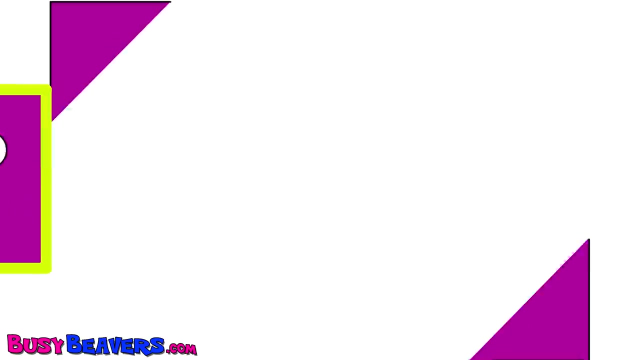 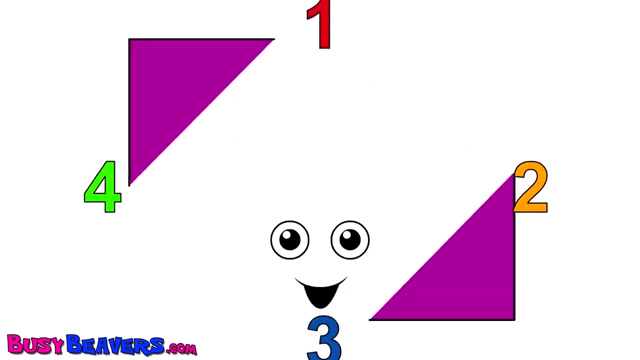 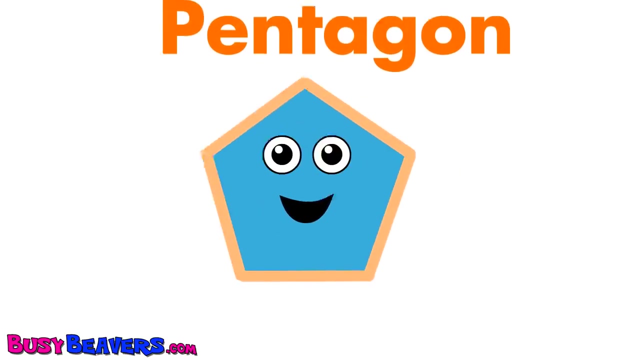 This little triangle has three sides: One, two, three sides. This little square has four sides. This little square has four sides. This little square has four sides: One, two, three, four sides. This little pentagon has five sides. 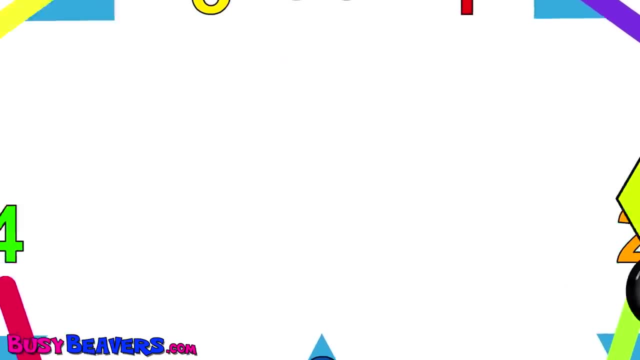 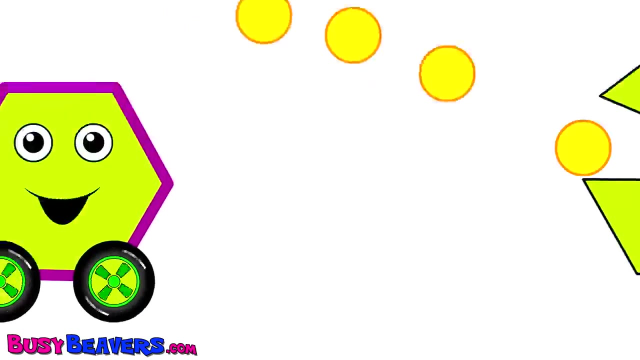 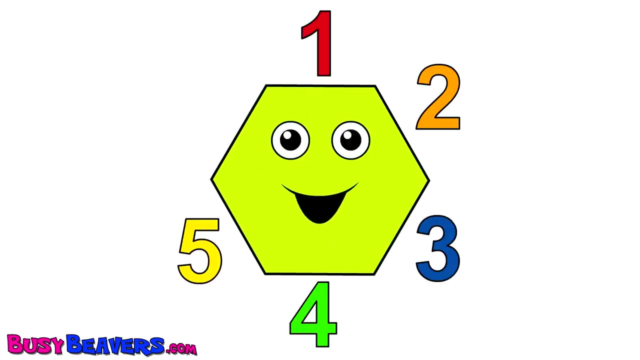 One, two, three, four, five sides. This little hexagon has six sides. This little hexagon has five sides, has six sides. This little hexagon has six sides: One, two, three, four, five, six. 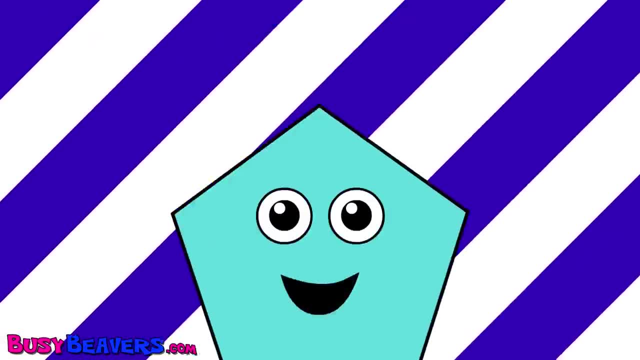 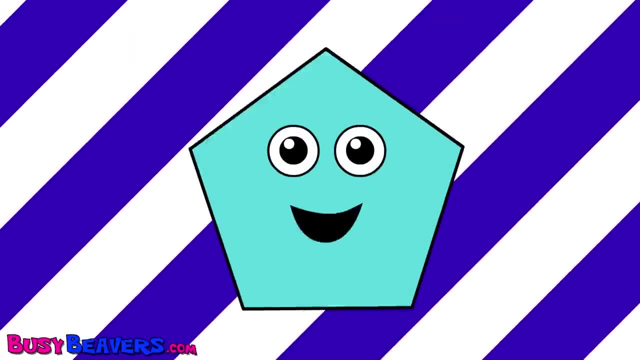 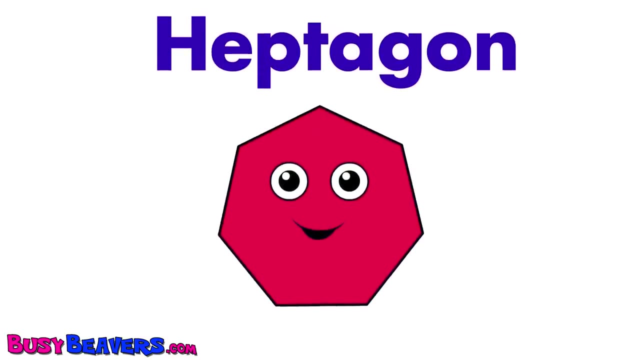 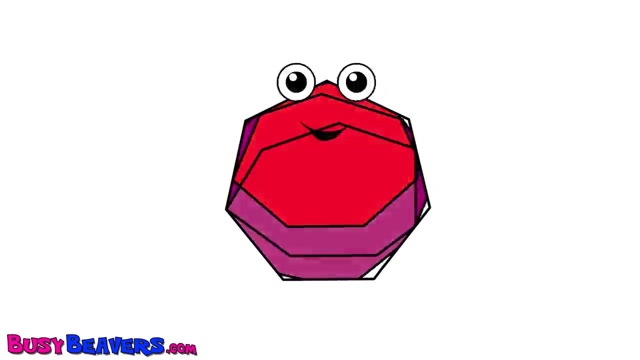 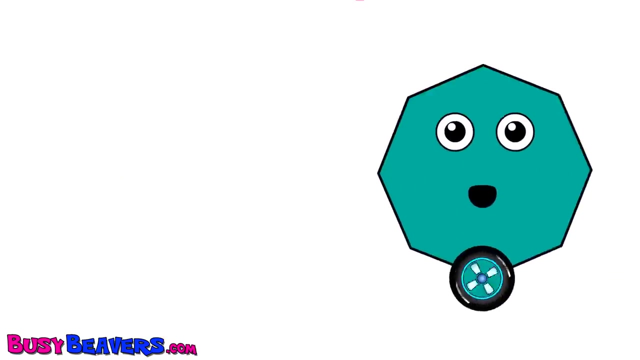 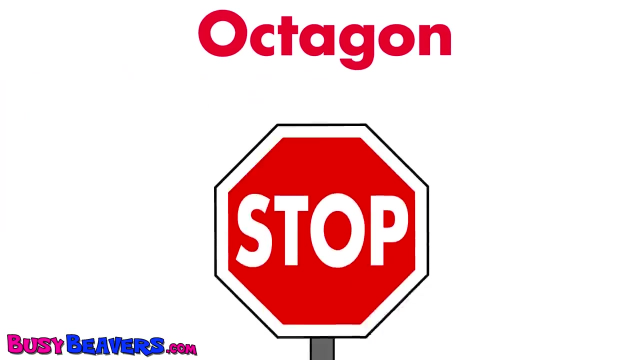 This little hexagon has seven sides. This little hexagon has seven sides. This little hexagon has seven sides: One, two, three, four, five, six. This little octagon has eight sides. This little octagon has eight sides. This little 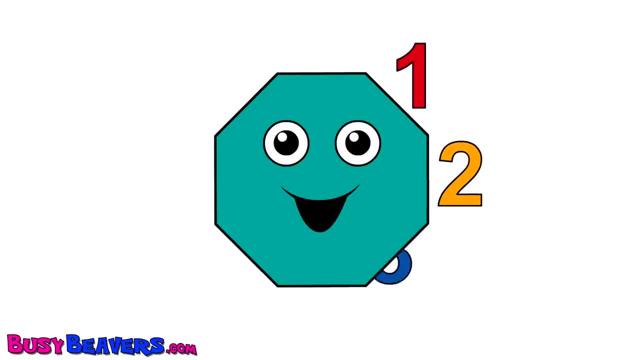 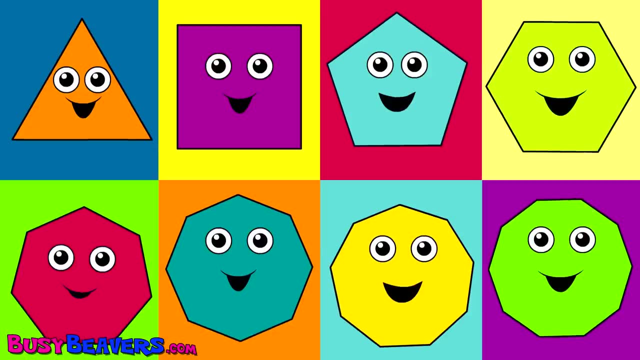 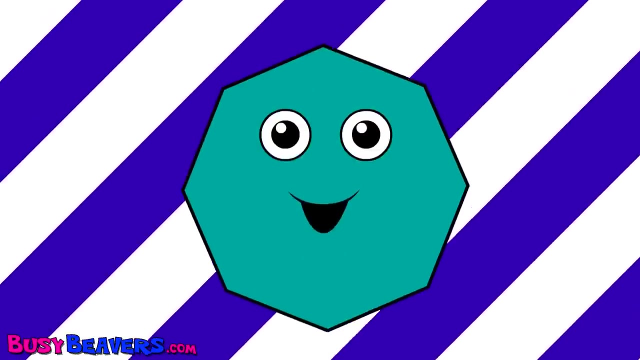 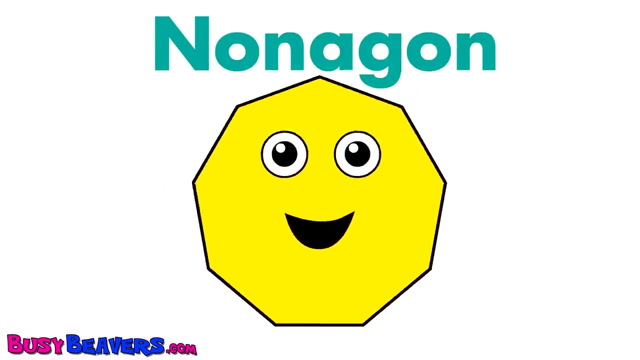 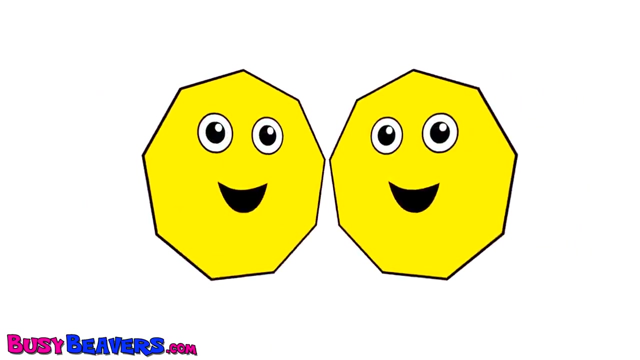 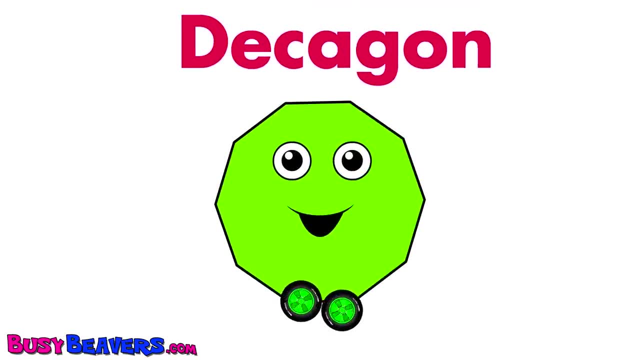 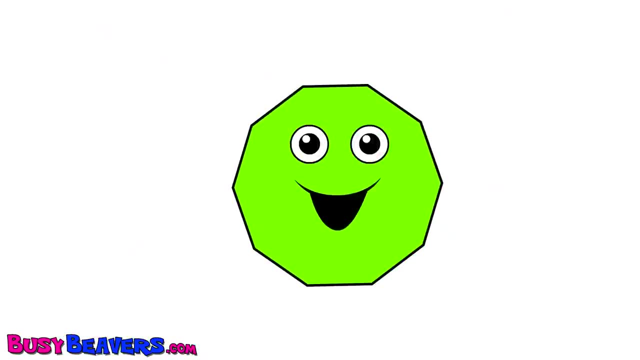 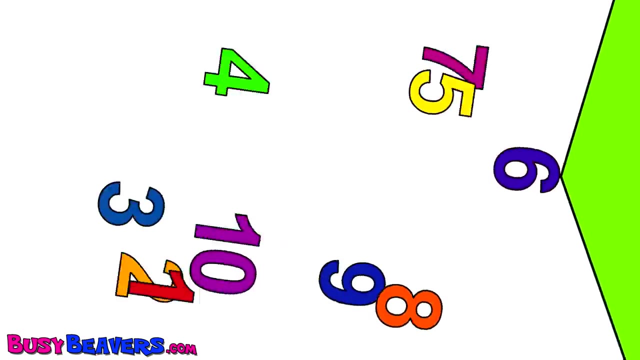 This little hexagon has ten sides. This little hexagon has ten sides. This little hexagon has ten sides: One, two, three, four, five, six, seven, eight, nine, ten. It's fun Yay. 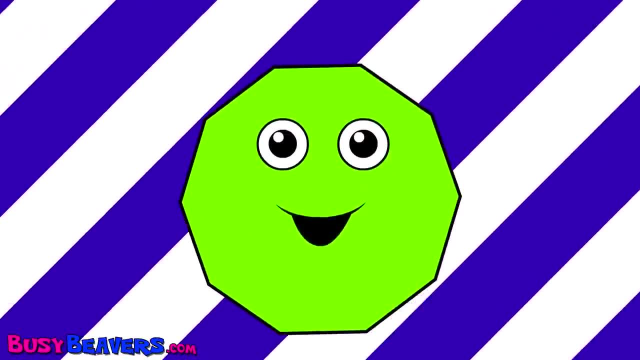 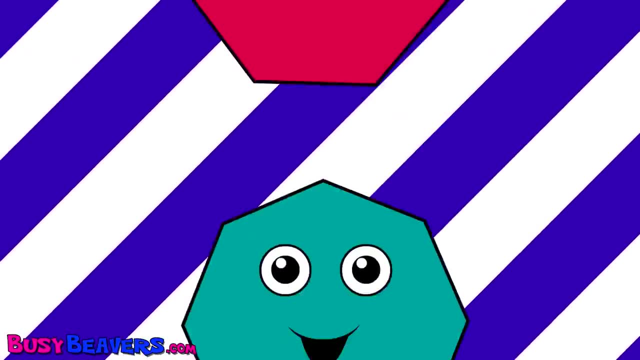 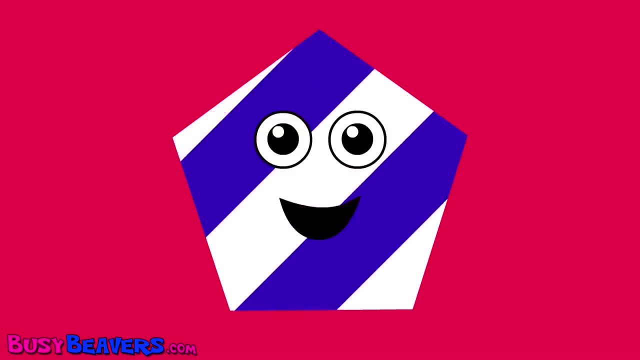 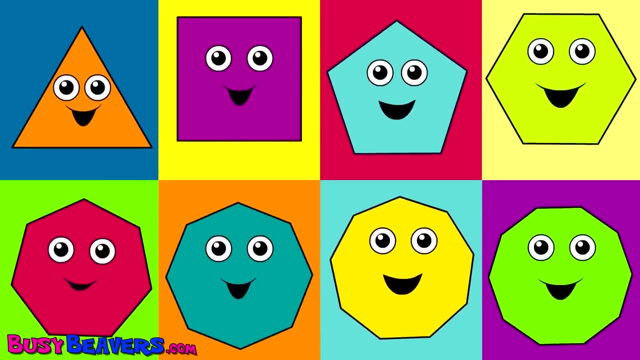 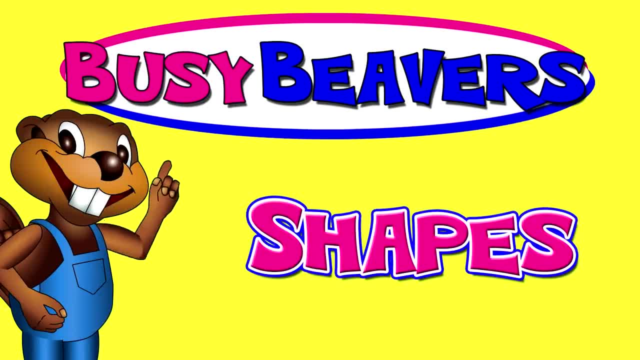 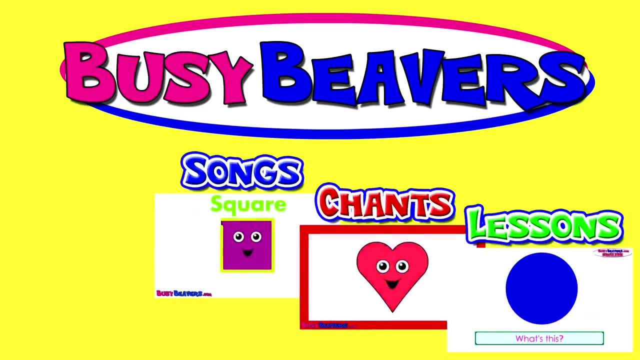 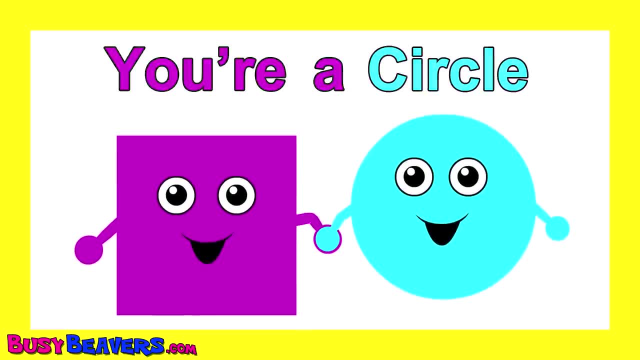 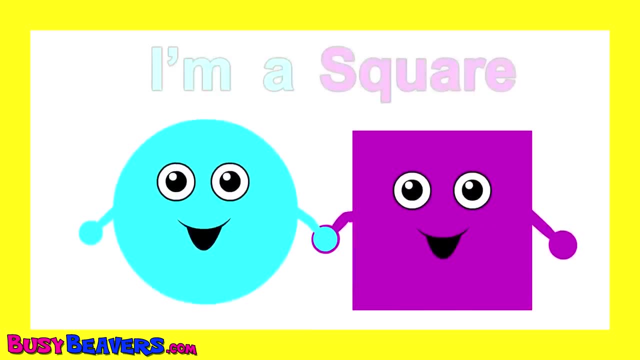 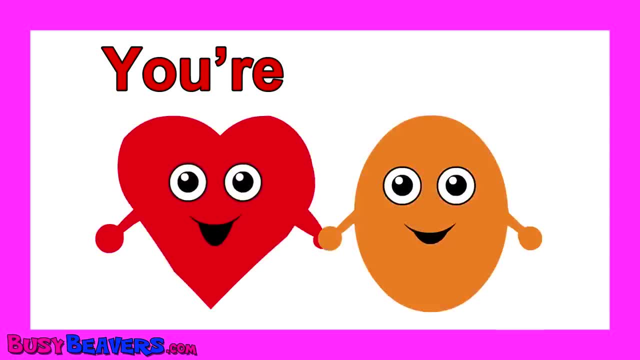 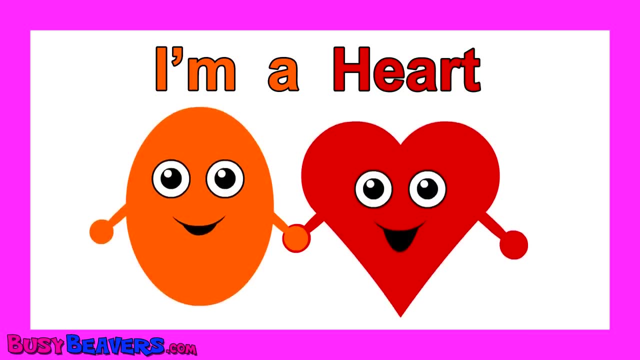 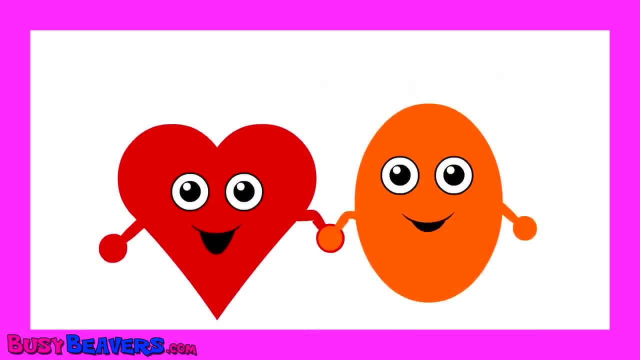 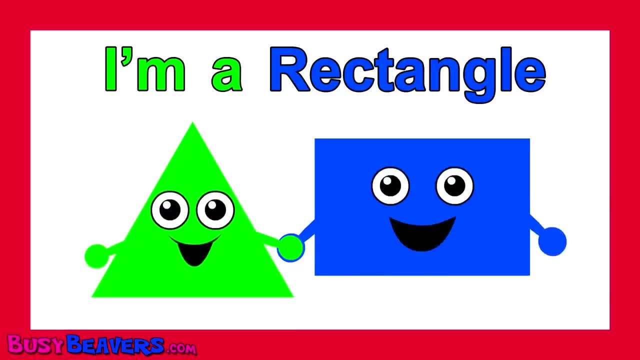 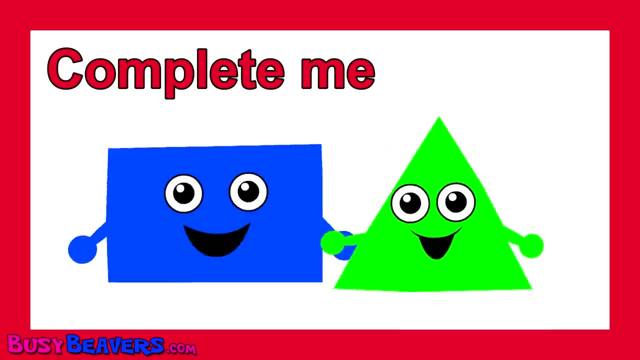 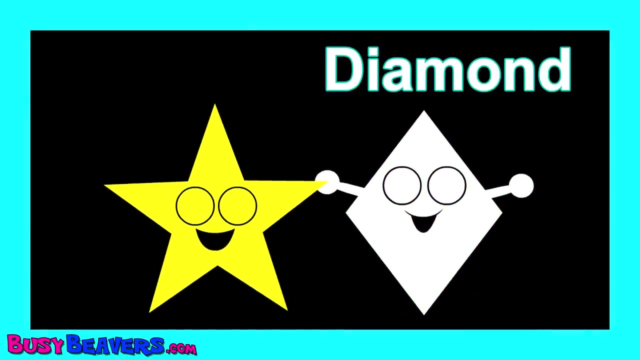 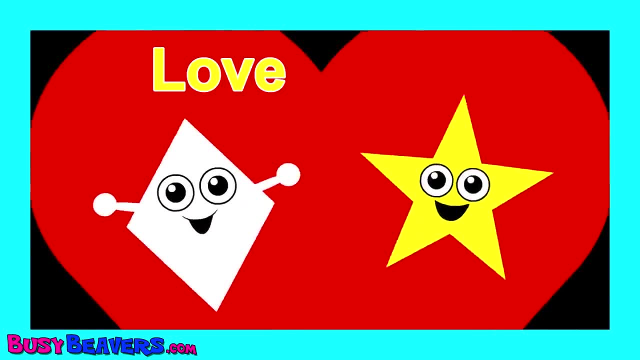 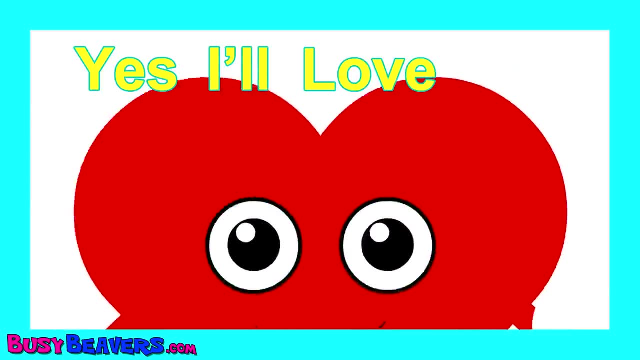 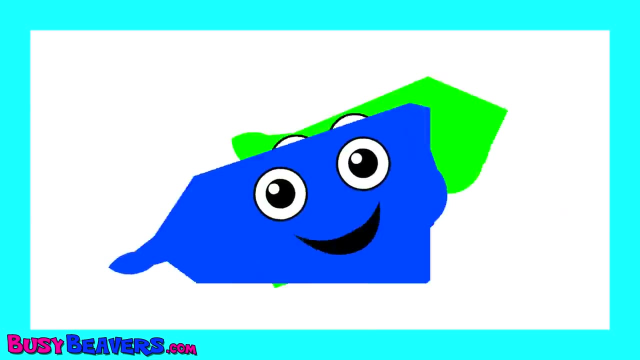 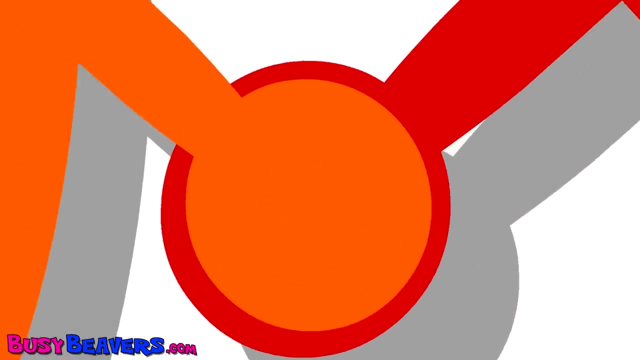 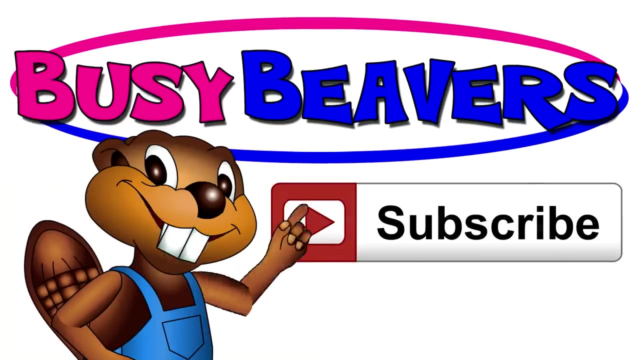 But I'll love you, love you, love you, whatever you are. Yes, I'll love you, love you, love you, whatever you are. When you subscribe to the Busy Beavers channel, you'll get a cool new song video like these every Monday: 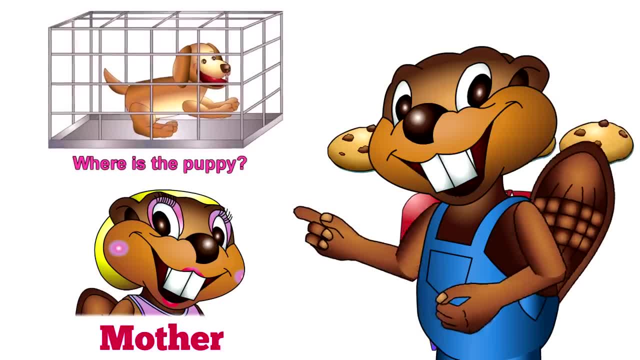 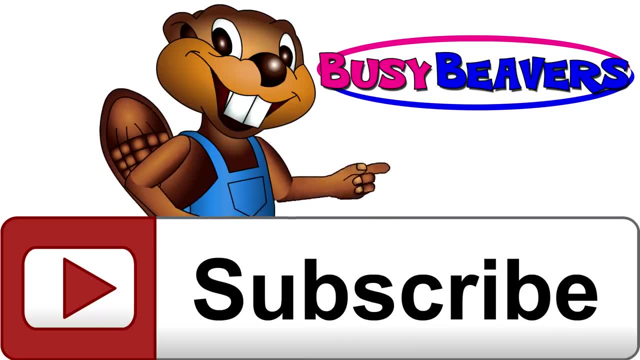 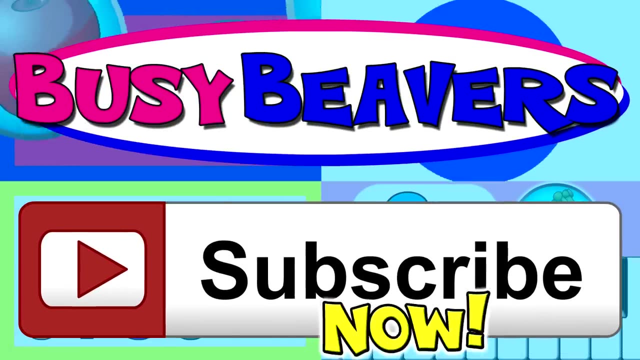 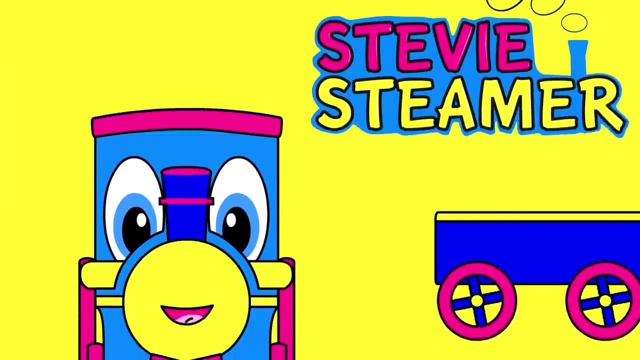 Or an educational, kindy lesson video like these. So what are you waiting for? Click that button to start learning and having fun And subscribe to Busy Beavers. Steamy Steamer- That's my name, Steamy Steamer. Hehe, I'm a turd. 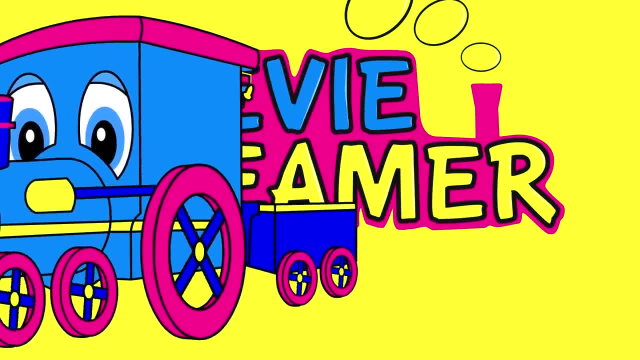 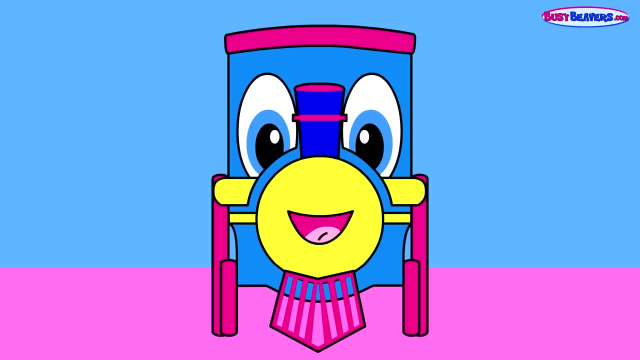 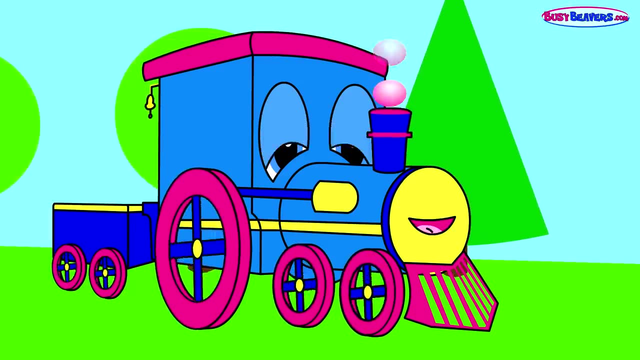 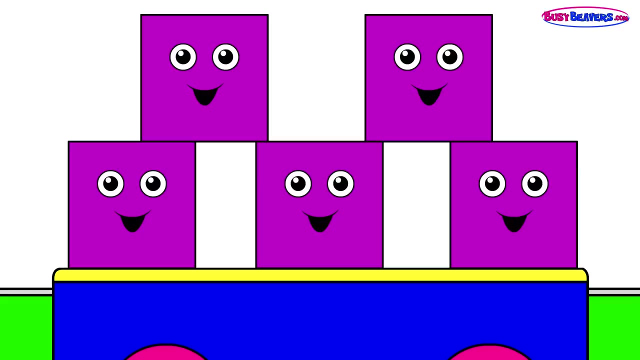 Hello, I'm Steamy Steamer. I'm a train. Today I'm pulling some more shapes. Let's go say hi to the shapes and count them: Squares, Squares One, two, three, One, two, three, four, five. 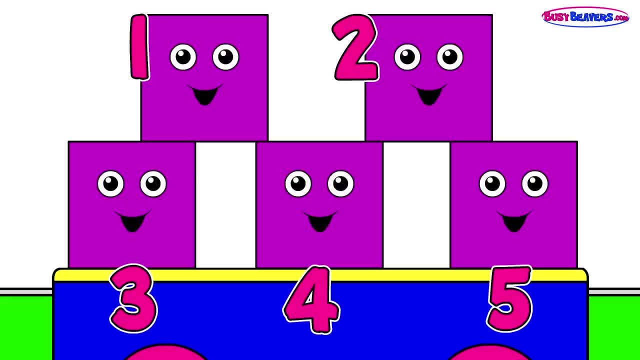 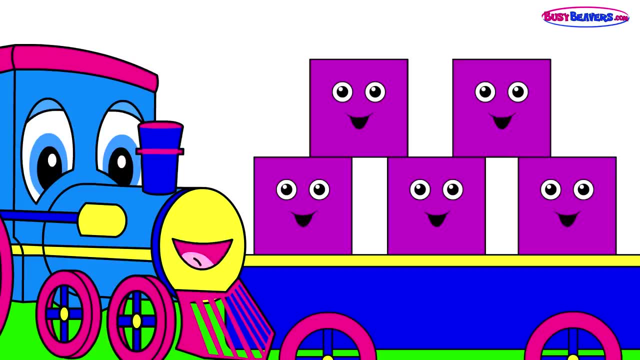 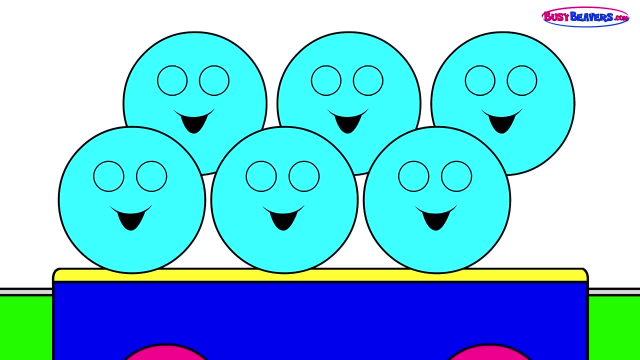 Five squares, Hi, squares, Hello, Hehe. so square Circles One, two, three, four, five, six Circles: One, two, three, four, five, six Circles, Hello, Six circles. 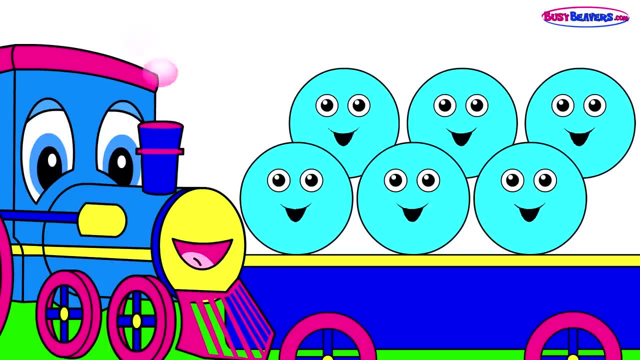 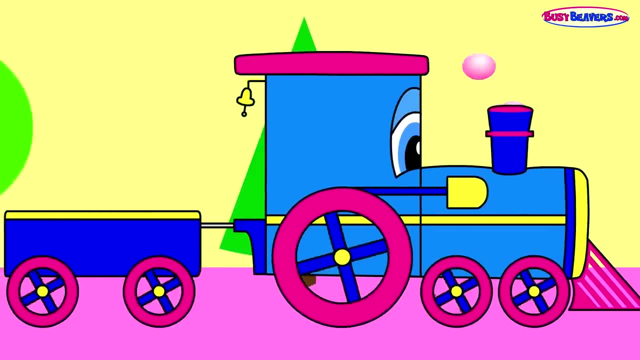 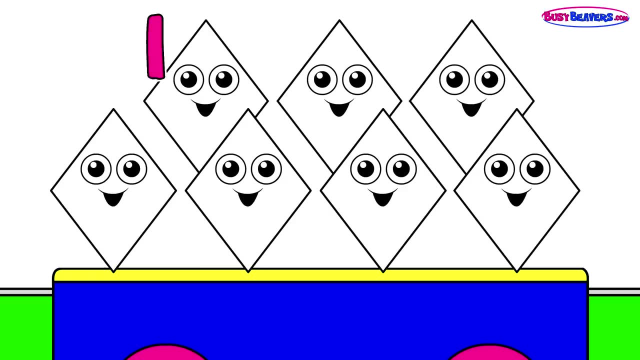 Hello circles, Hello circles, Hi, Hello, Stevie Steamer, Hi Hi, Nice shapes, Hey, Nice shapes. Nice shapes, I mean the people are identify with us though. Diamonds One, Two, Three. 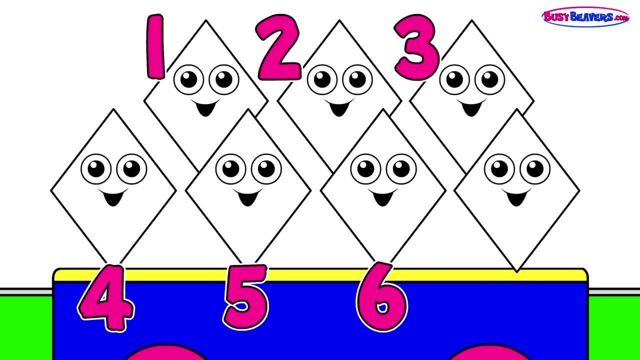 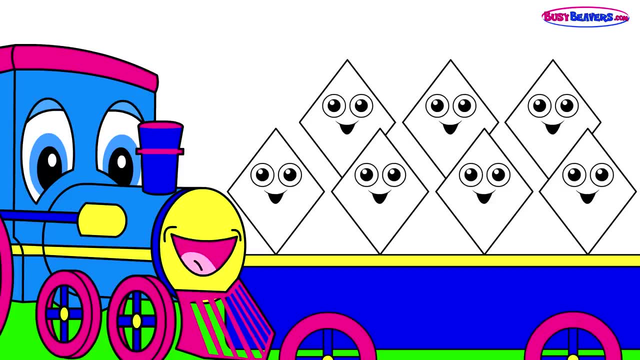 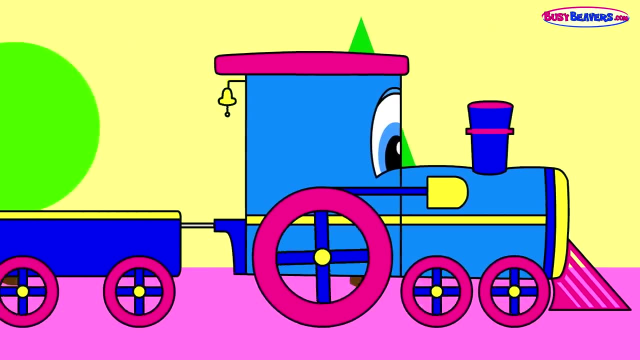 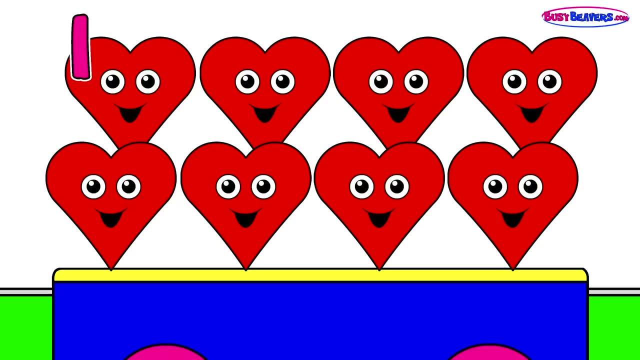 Four, Five, Six, Seven, Seven Diamonds, Seven diamonds, Hi diamonds, Hi Stevie, Looking sharp Hearts. One, two, three, four, five, six, seven, eight, Eight hearts, Hello hearts. 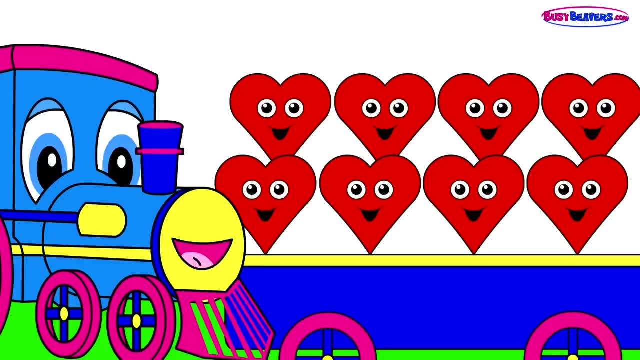 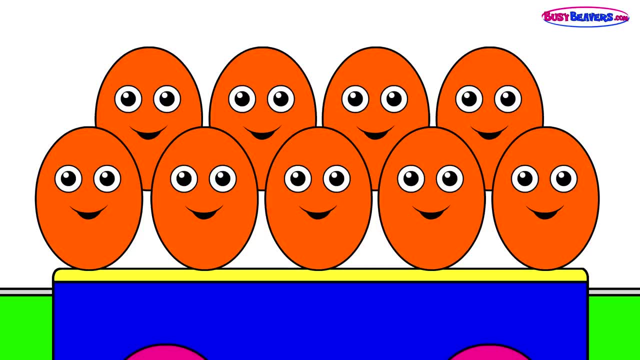 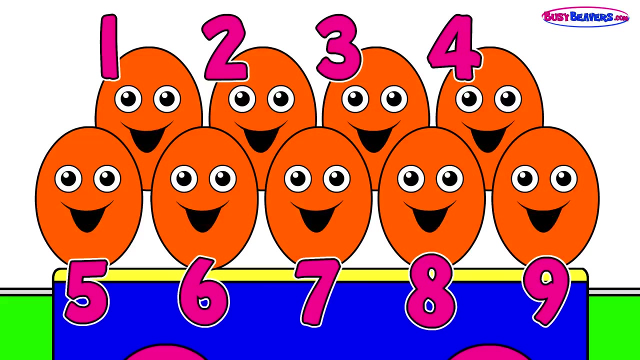 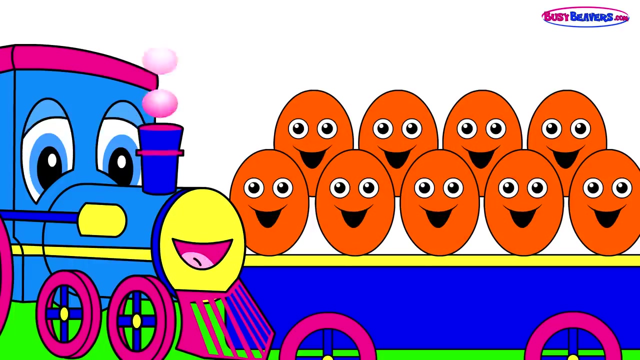 Hello, Hey, how you doing Hearts, I love them. Ovals One, two, three, four, five, six, seven, eight, nine, Nine ovals, Hi, ovals, Hi, Stevie Steamer. 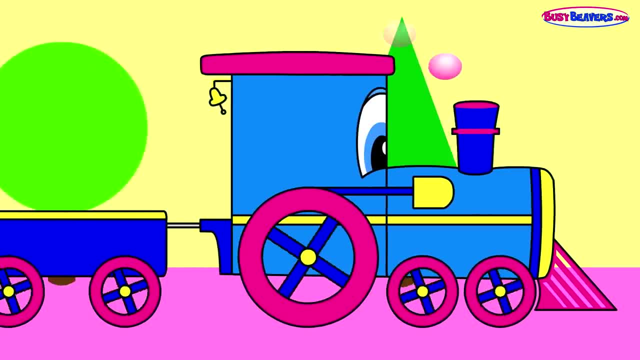 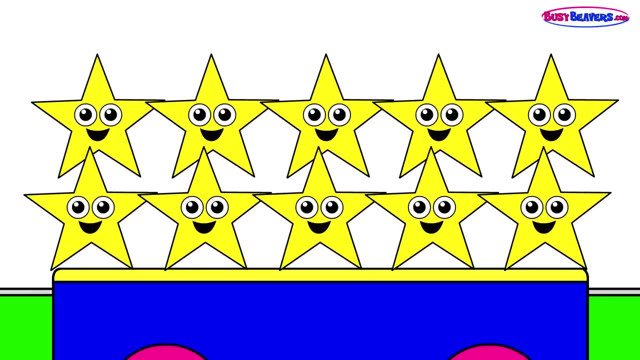 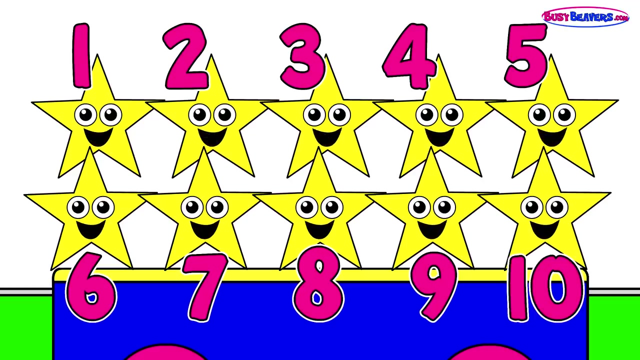 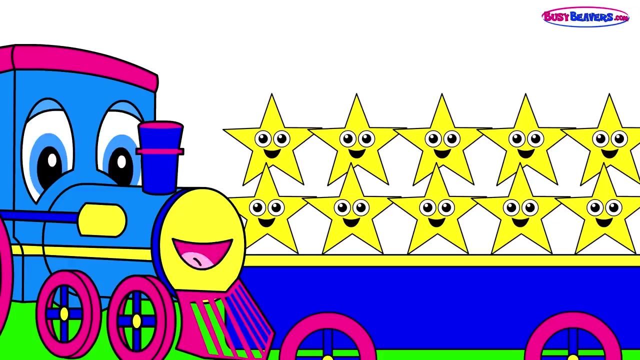 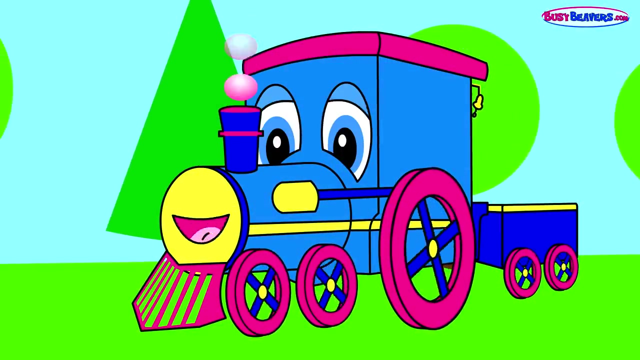 So round. Stars One, two, three, four, five, six, seven, eight, Nine, ten Ten. stars Hi, stars Hi, Stevie, Very sparkly, Very twinkly. Well, that's all the shapes for today. 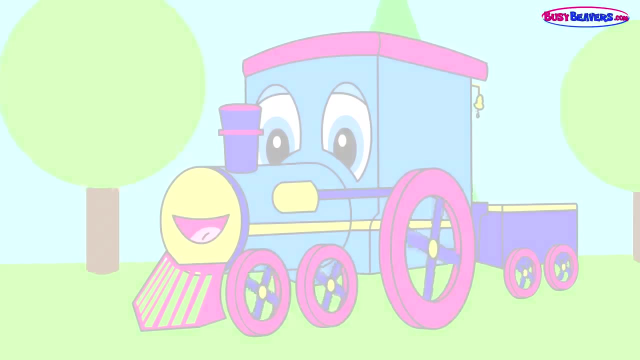 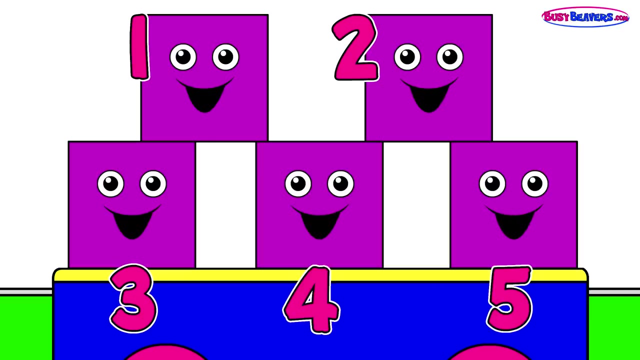 Let's count them one more time: One, two, three, four, five squares. One, two, three, four, five squares. One, two, three, four, five, six circles: One, two, three, four, five, six, seven diamonds. 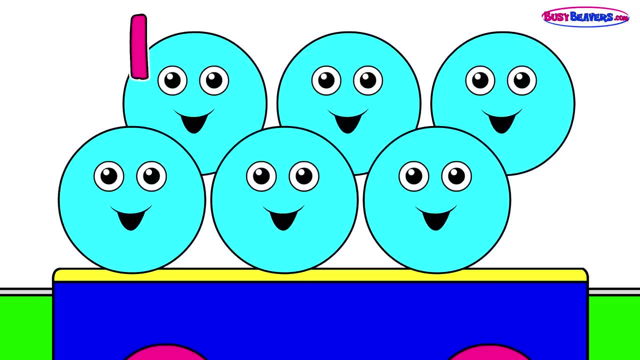 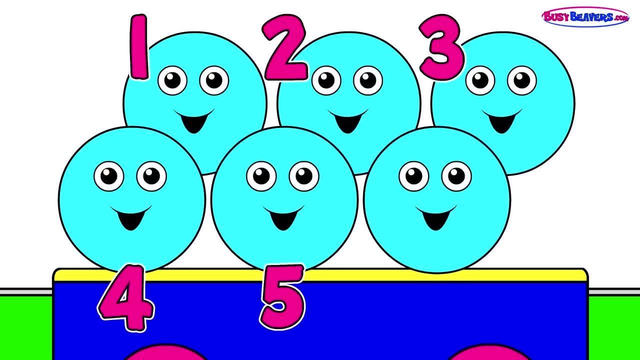 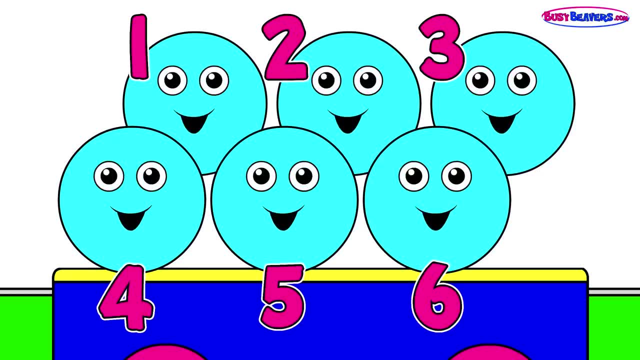 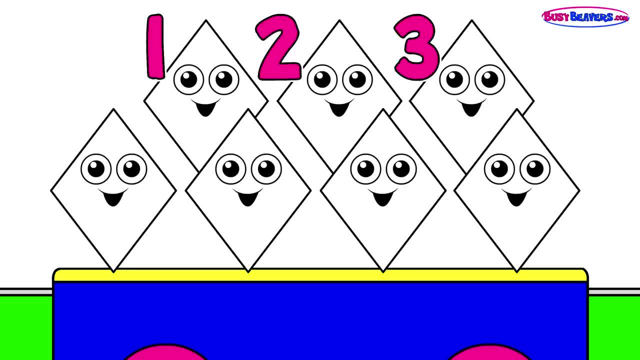 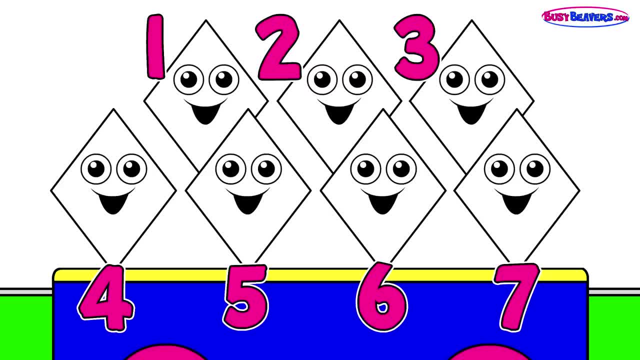 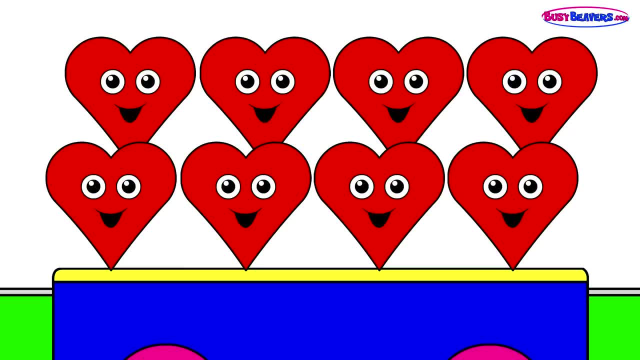 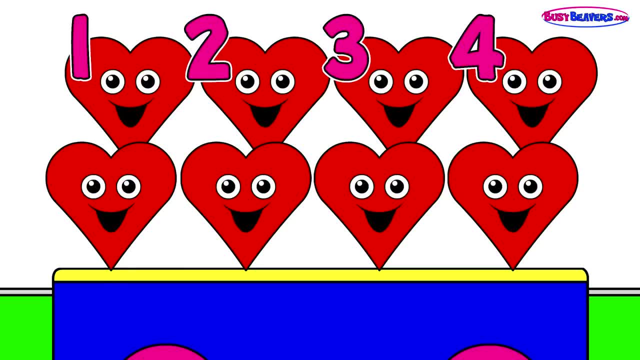 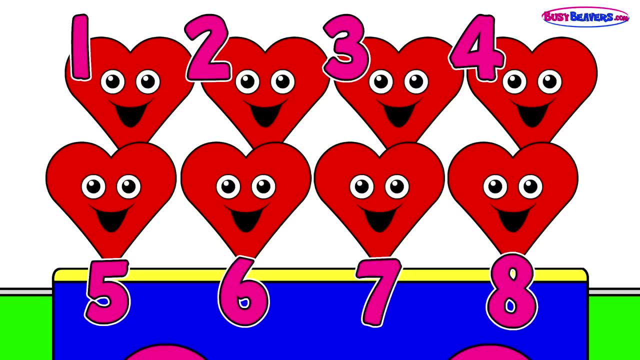 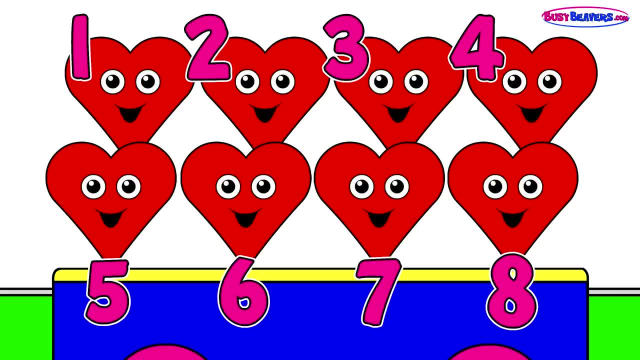 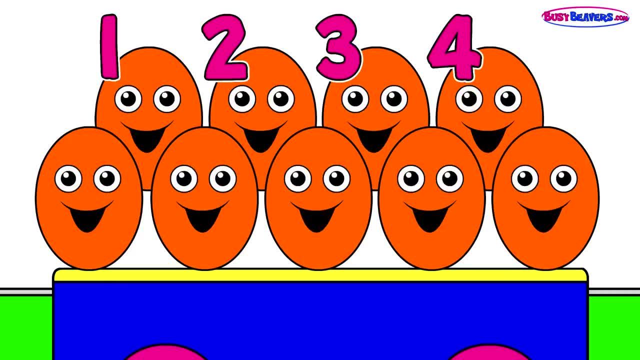 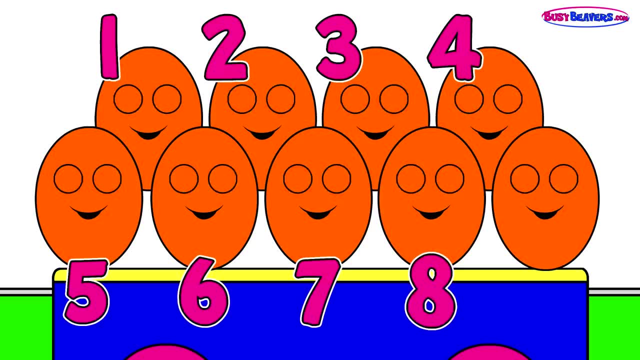 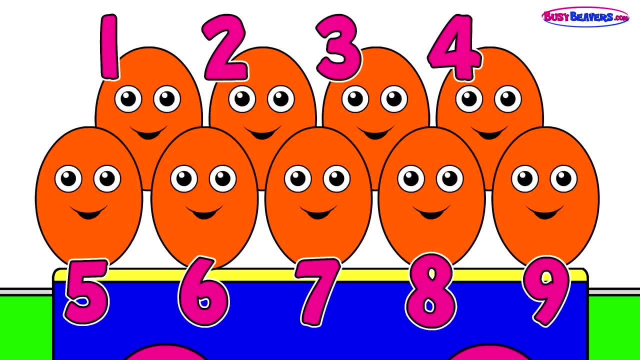 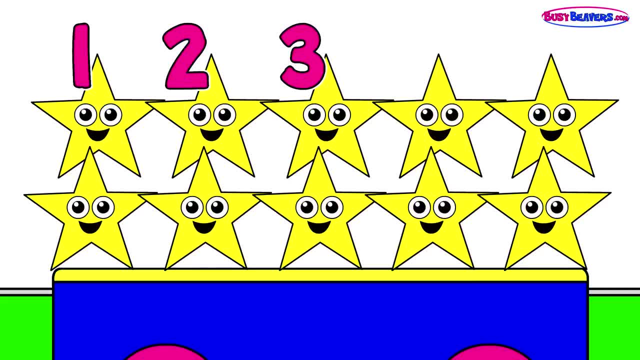 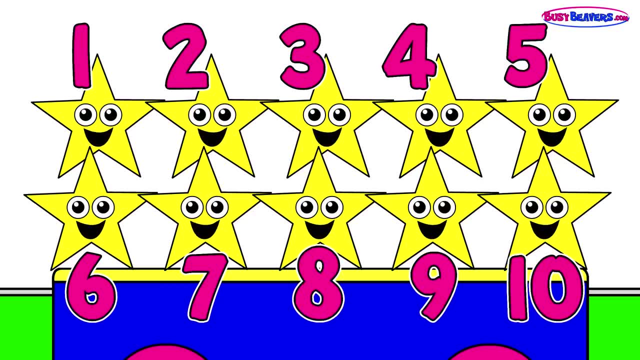 One, two, three, four, five, six, seven diamonds. One, two, three, four, five, six seven diamonds. One, two, three, four, five, six, seven, eight, nine, ten stars. 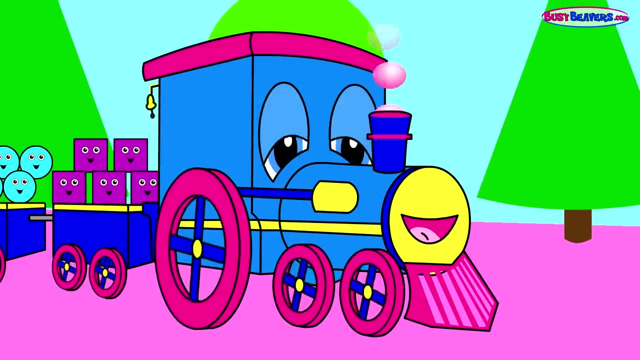 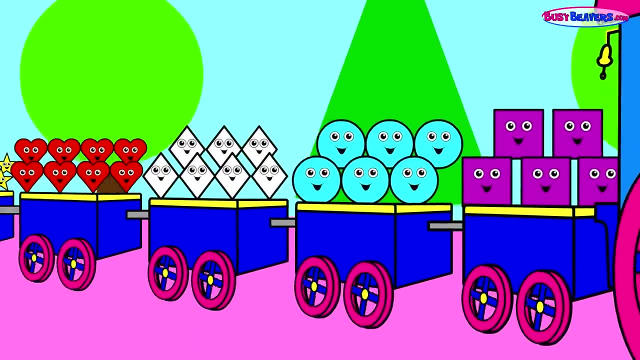 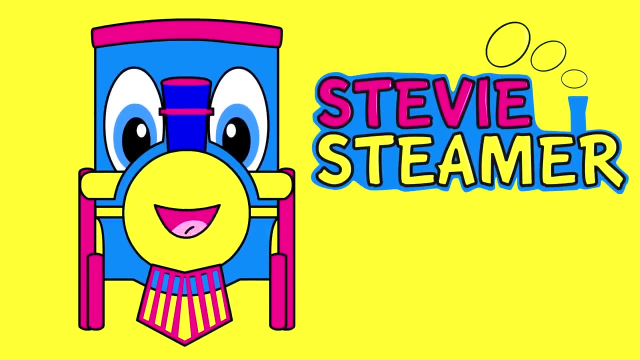 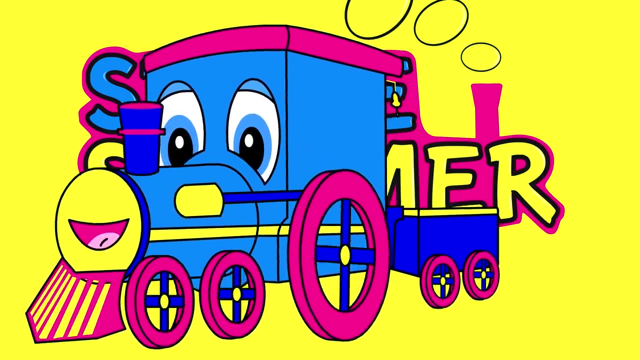 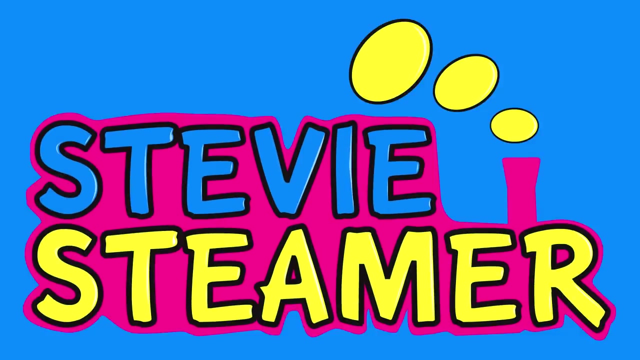 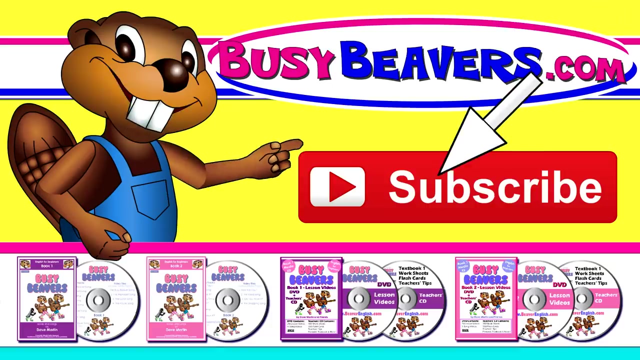 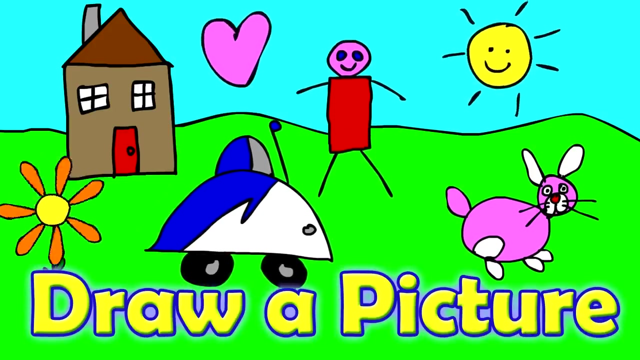 All aboard, Here we go. Steady steamer, That's my name. Steady steamer, That's my name. Stevie Steiner, I'm a train Draw, a rectangle With a circle on top, To her arms, to her legs. 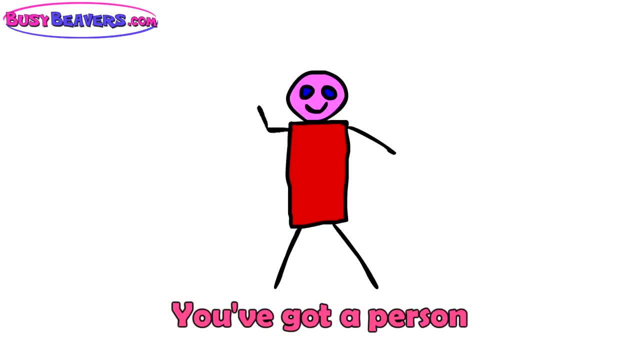 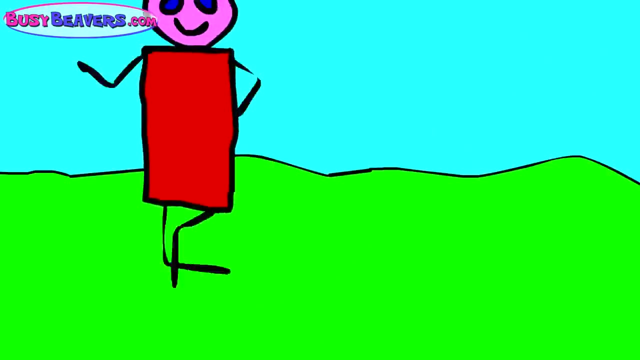 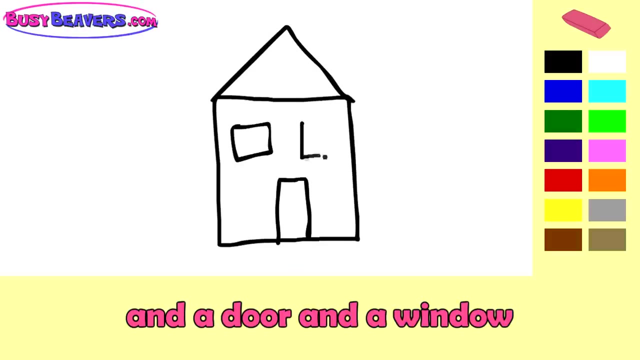 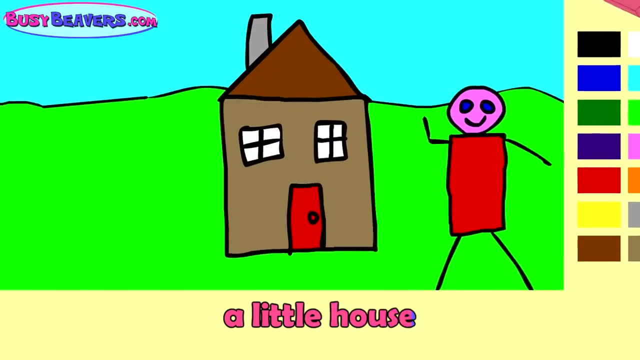 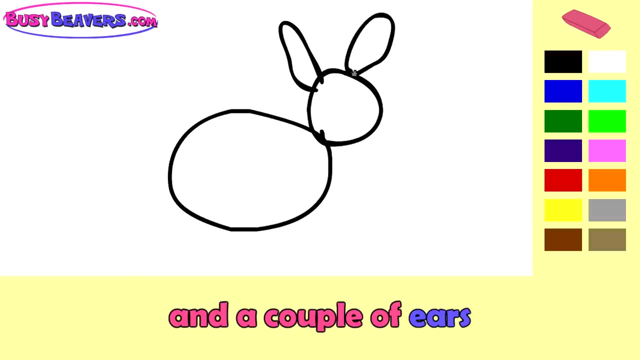 What have you got? You've got a person, A happy person. Draw a square With a triangle top And a door and a window. Hey, what have you got? You've got a house, A little house. Draw an oval And a circle And a couple of ears. 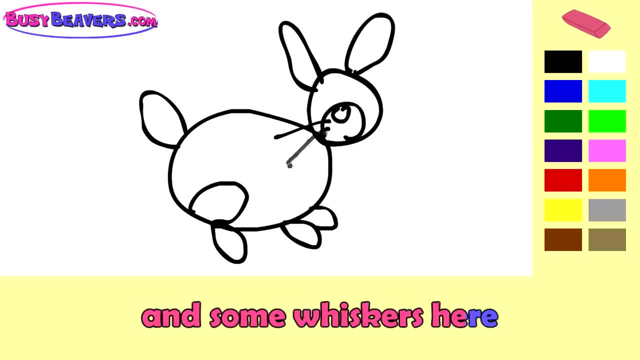 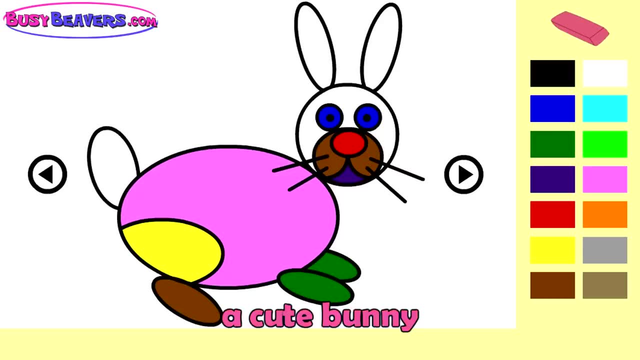 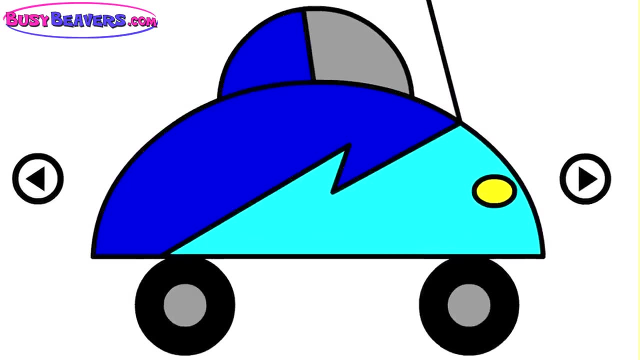 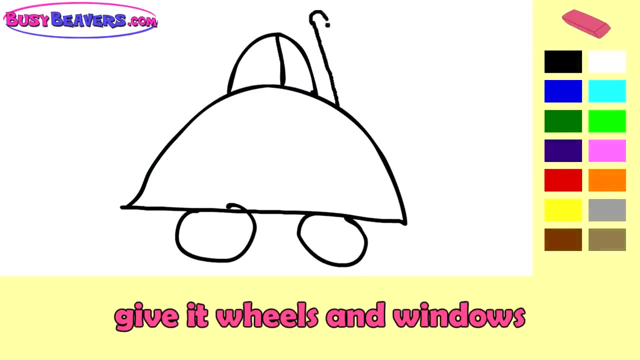 A tail, feet, a face And some whiskers. Here you've got a bunny. Look at that. A cute bunny Draw a half circle With another on top. Yeah, and we are A circle and a window. Hey, what have you got? You've got a car. 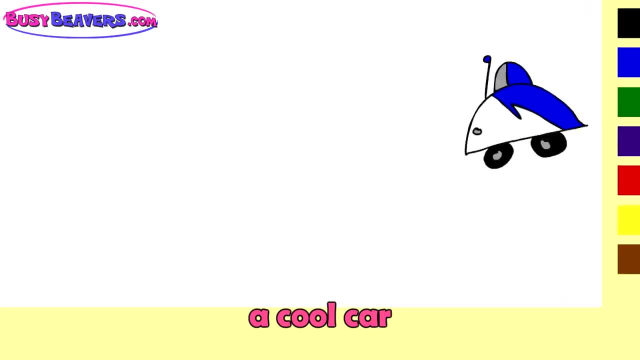 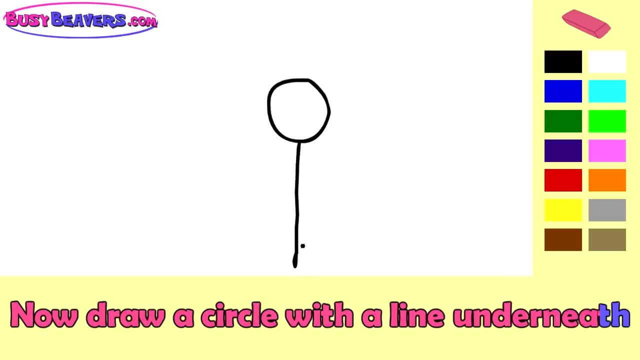 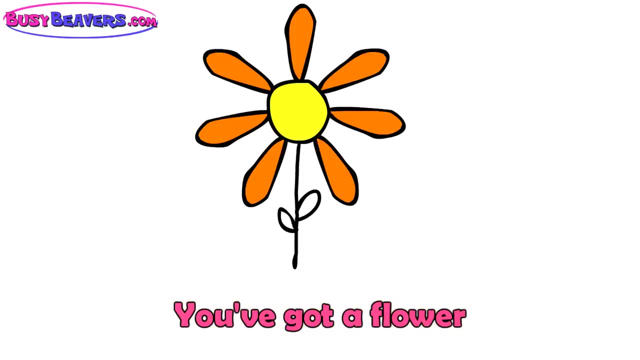 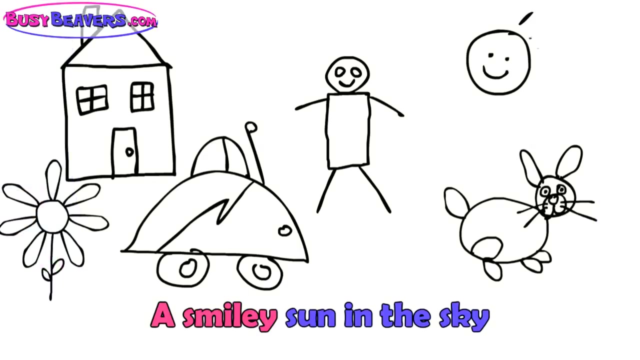 A cool car. Now draw a circle With a line underneath A bunch of ovals. Four petals And two four leaves. You've got a flower, A pretty flower, A smiley face And a smiley face, A smiling sun in the sky And a heart-shaped cloud And a swiggle through the mill. 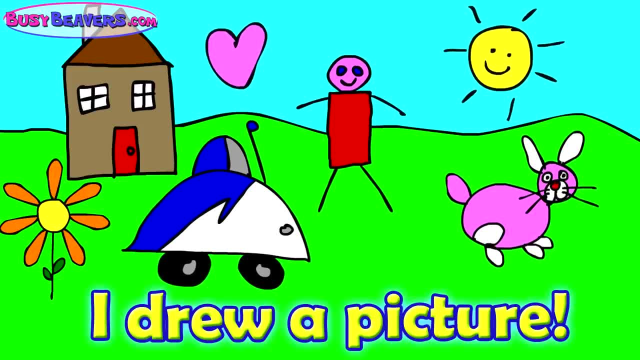 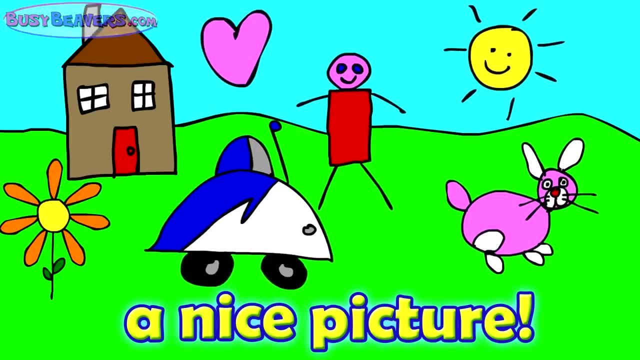 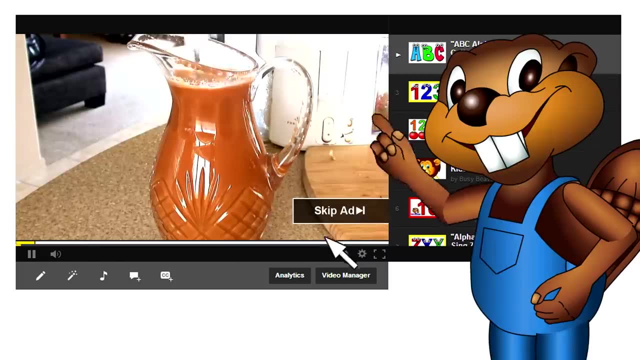 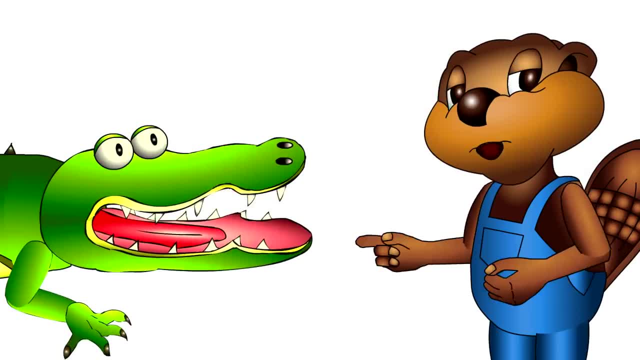 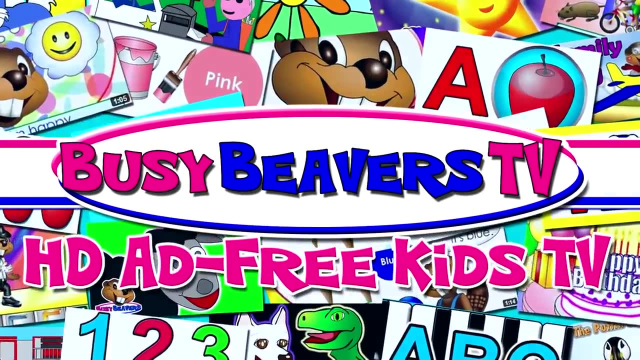 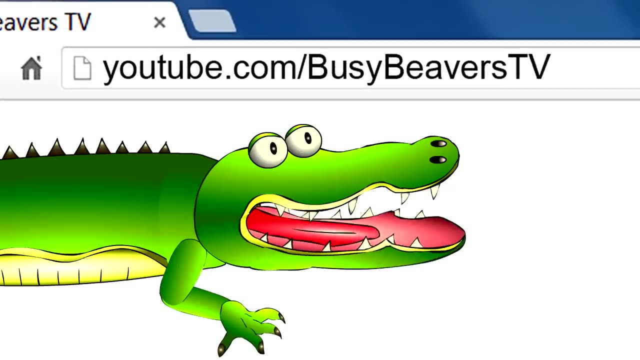 Oh, they're very, Very frustrating. I know Well, Busy Beavers have a new channel, Busy Beavers TV, where all of our kids' learning videos are in HD and ad-free. So let me get this straight: YouTubecom slash. Busy Beavers TV has all of the Busy Beavers song videos. 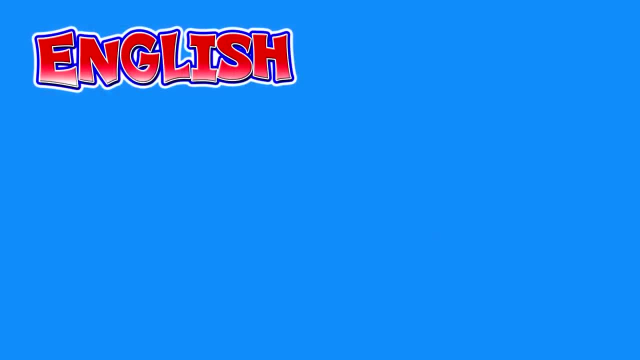 Yeah, And all of the kindy lesson videos. That's right, And I can learn to speak English, Chinese, Korean, Spanish and more. Yes, And there's no ads, No ads, No pop-ups, No pop-ups. 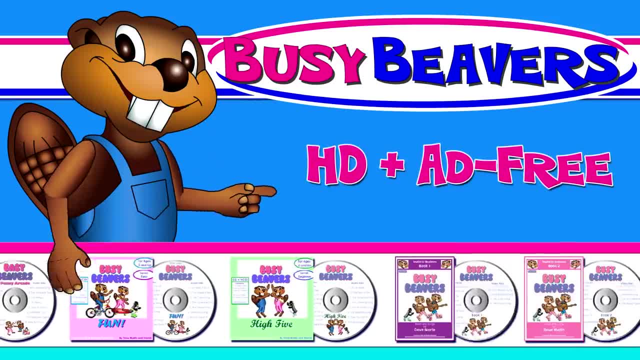 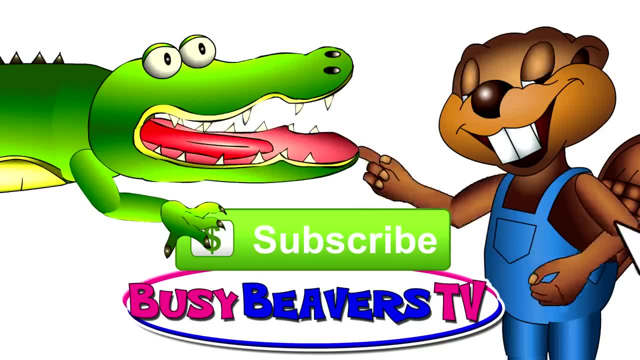 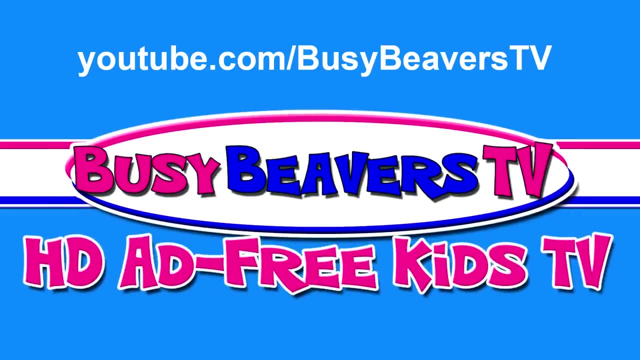 And no commercials. All of the great content from our free channel in HD and ad-free. That's it. I'm clicking that button and I'm not kidding. Do it. YouTubecom slash. Busy Beavers TV for kids' learning videos in HD and ad-free. 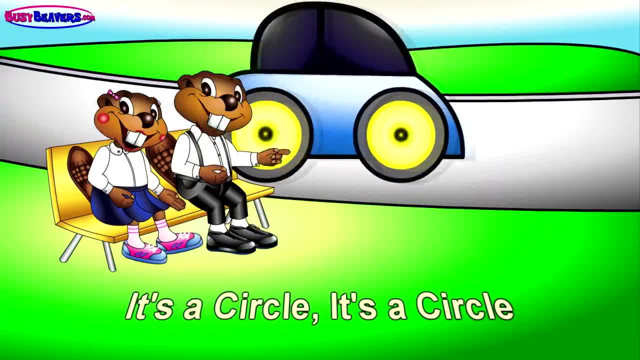 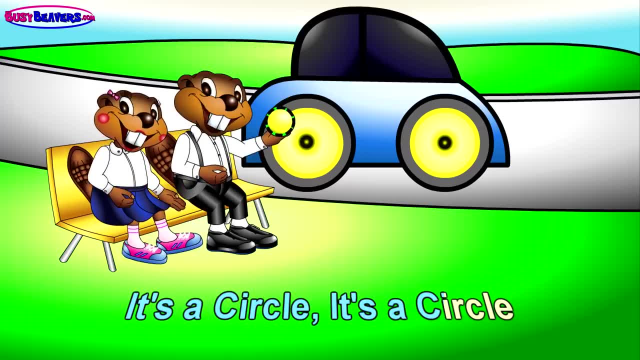 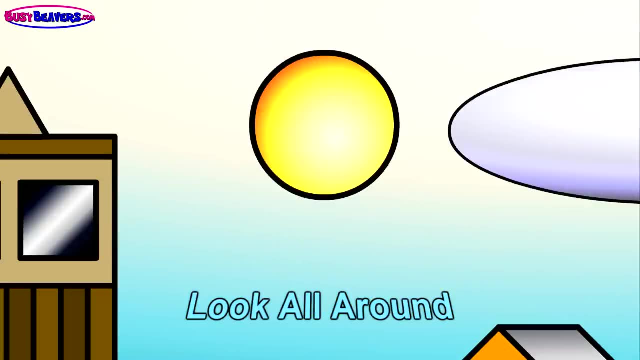 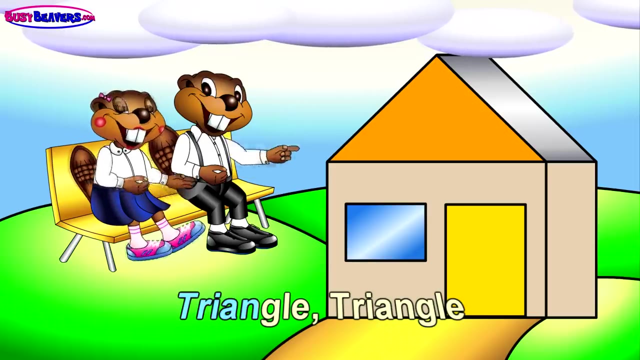 It's a circle, it's a circle. a circle is round. It's a circle, it's a circle, a circle is round. Look up and down, look all around. do you see circles? Triangle, triangle one, two, three. 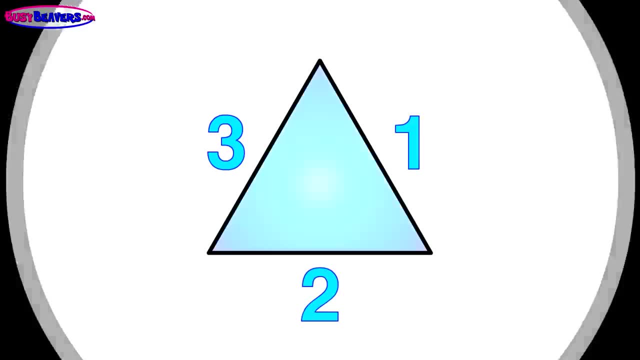 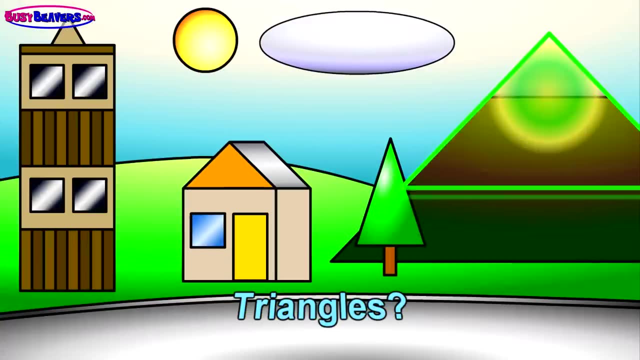 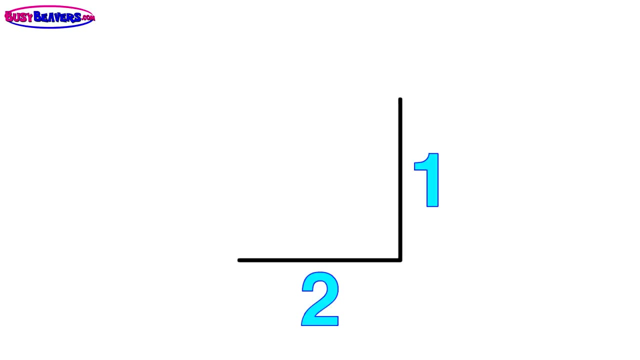 Triangle, Triangle, triangle. one, two, three. Look all around you. can you see triangles? It's a square. it's a square. one, two, three, four. It's a square. it's a square: one, two, three, four. 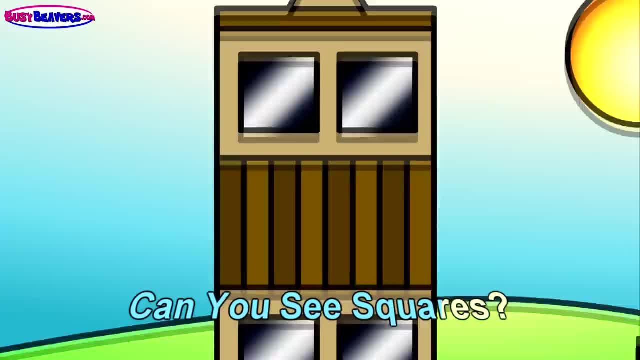 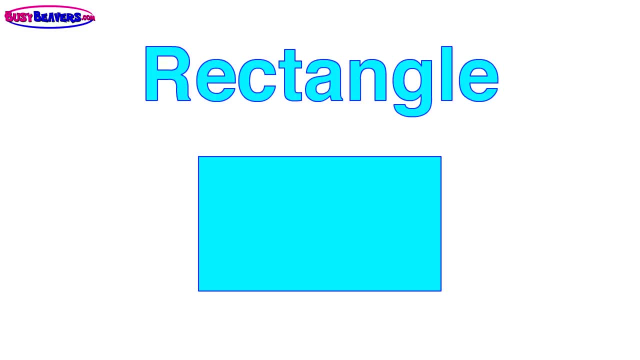 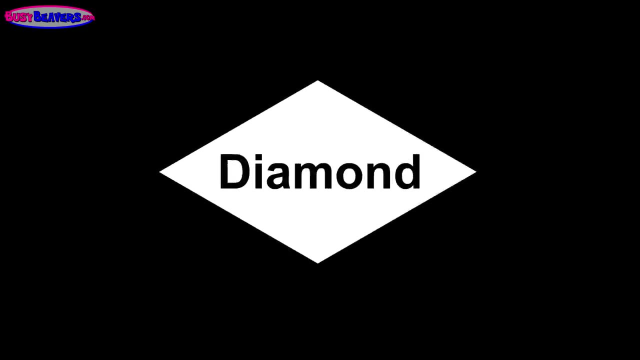 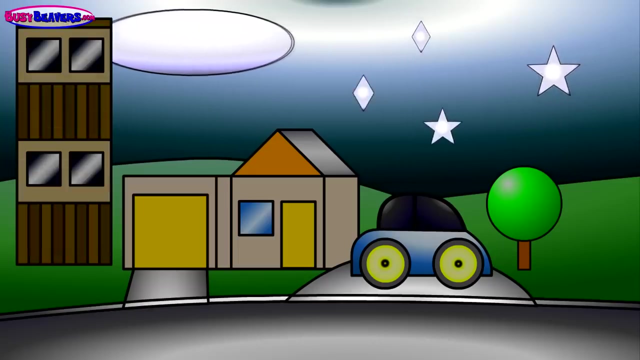 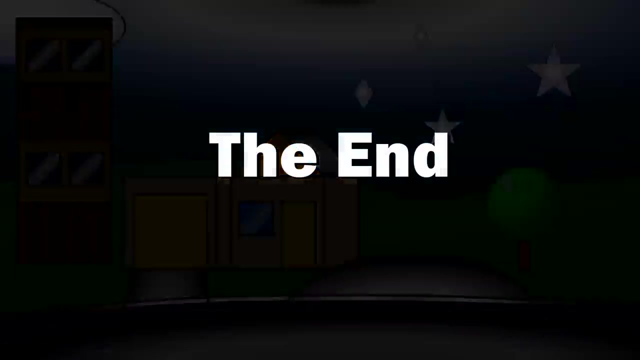 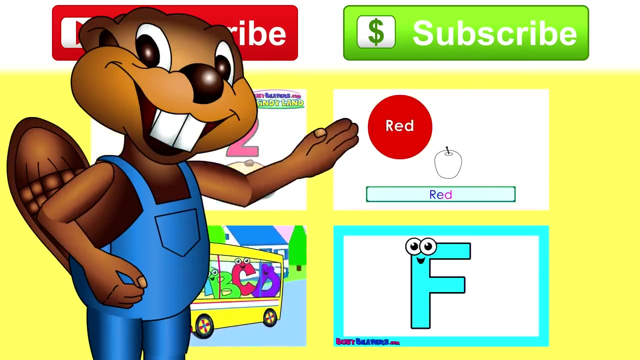 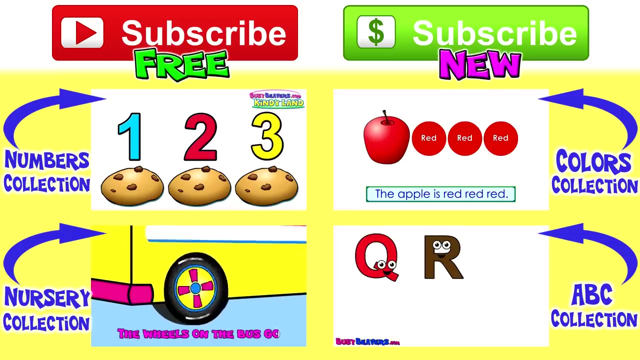 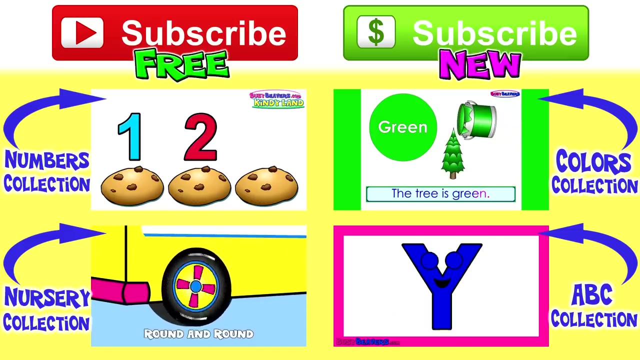 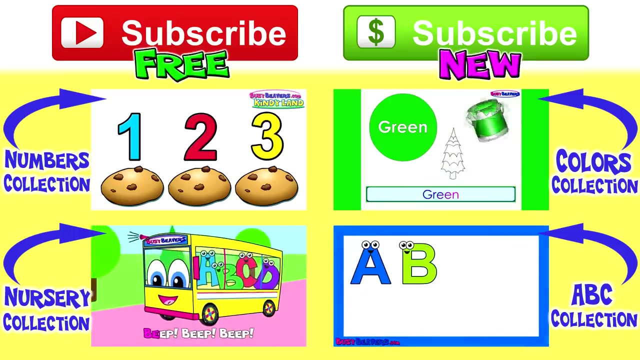 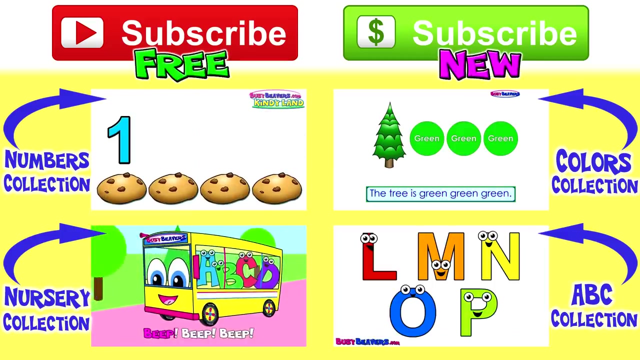 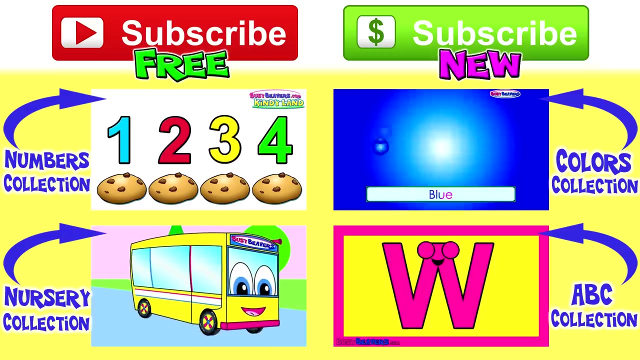 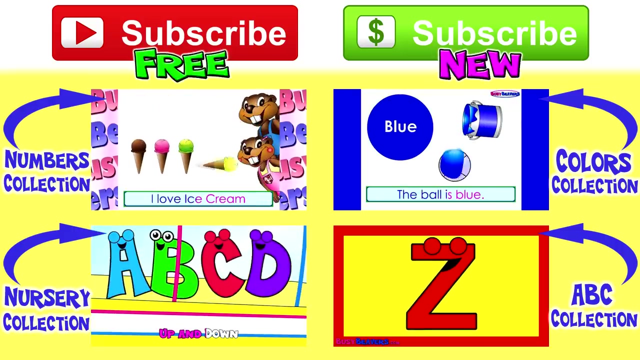 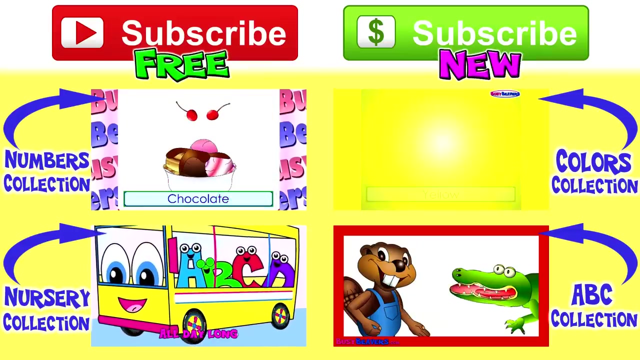 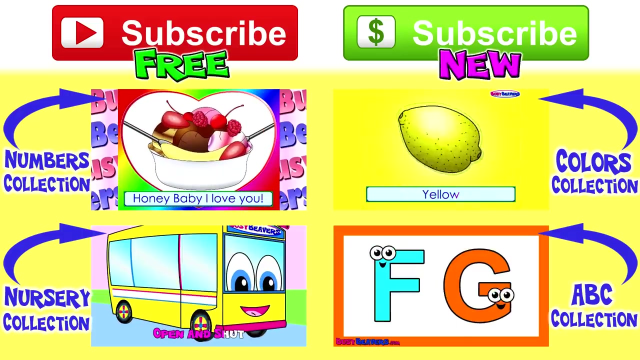 Look over there. can you see squares? I see squares. Rectangle oval diamond star. Rectangle oval diamond star. Rectangle oval diamond star. these other cool Busy Beavers videos. Thanks for watching. Thanks for watching.